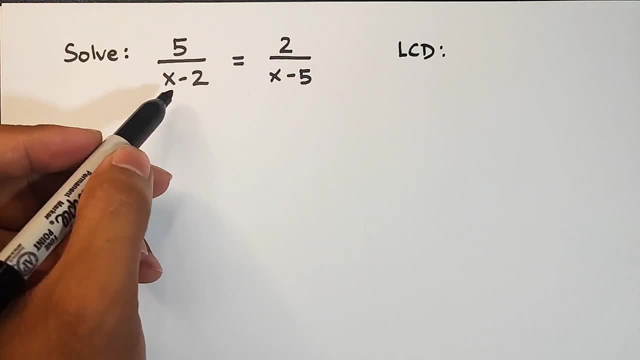 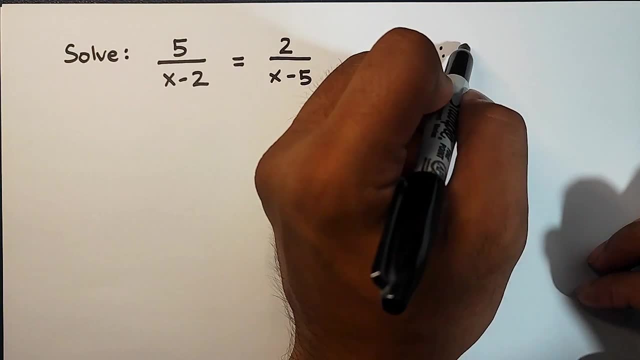 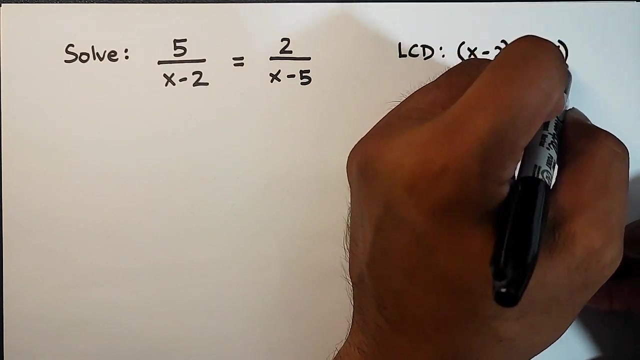 denominators x minus 2 and x minus 5.. So if you want to determine the LCD of these two denominators, simply express them as factors, like this: one x minus 2 times x minus 5.. So, as you can see, we expressed it as factors, but you don't. 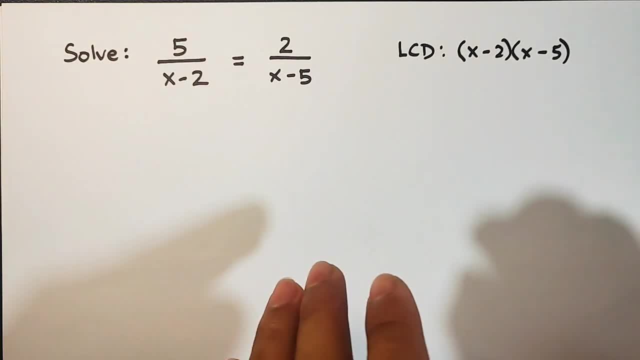 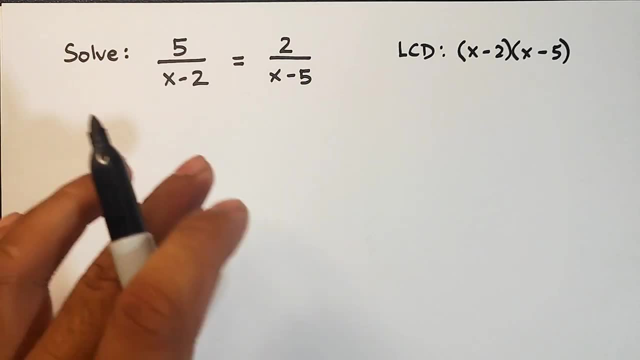 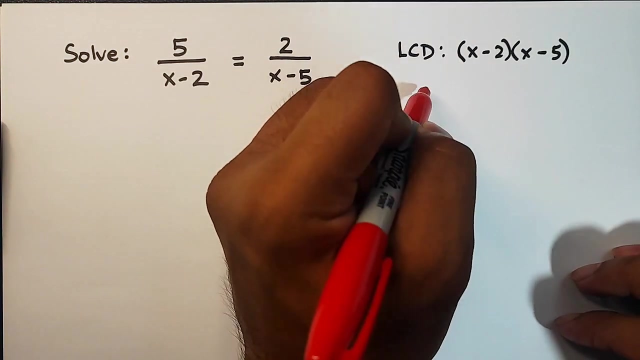 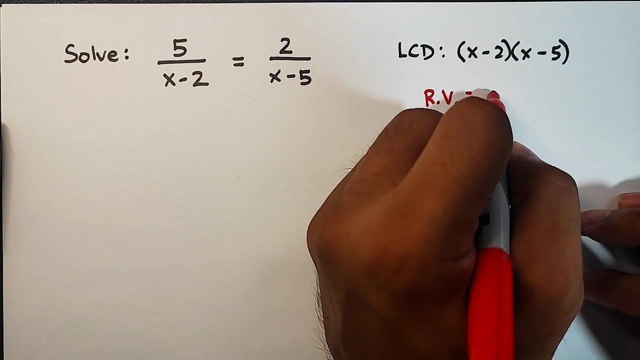 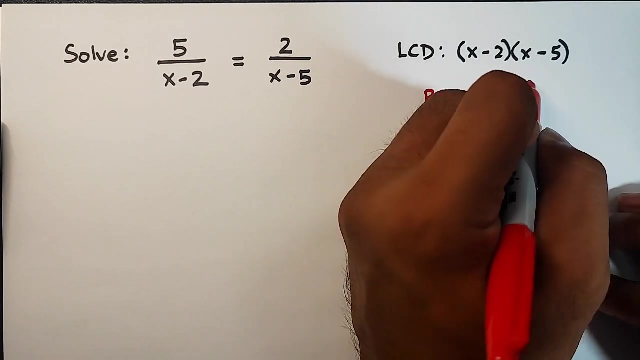 need to multiply it. So it is x minus 2 times x minus 5.. And, by the way, guys, before we proceed in solving this equation, let's identify our restricted value. Our restricted value for RV is positive 2 and positive 5.. So why is the restricted value of 2 and positive? 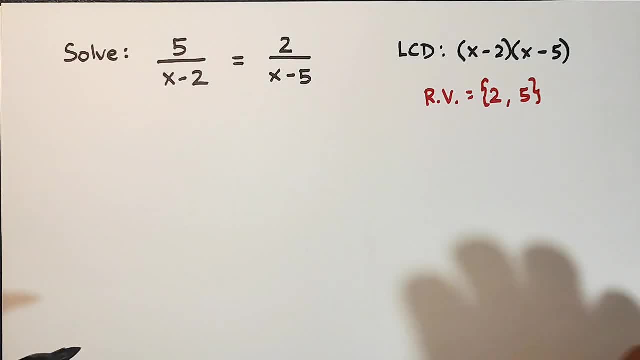 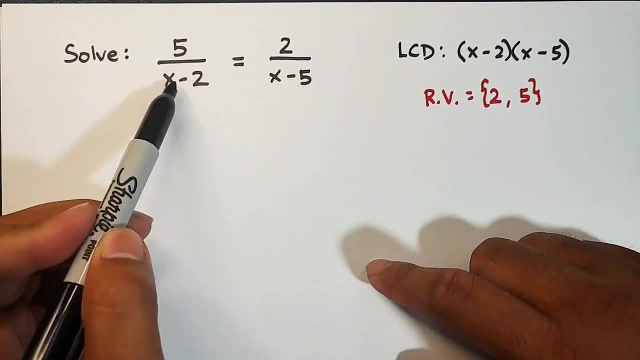 5?. What this means is that they cannot be the value of x, because it will cause your denominator to be equal to 0. Imagine, when you substitute the value of x as 2, that is, 2 minus 0, it will become undefined. Same with positive 2 and positive 5.. So if you 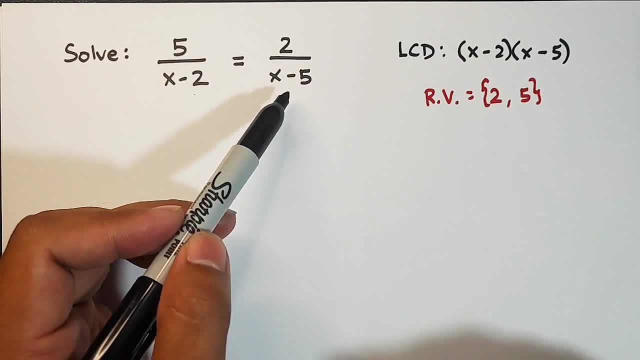 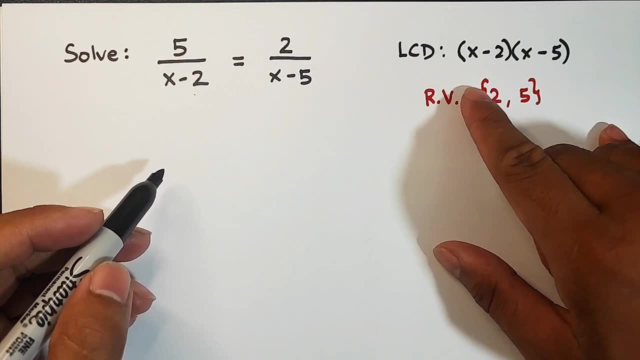 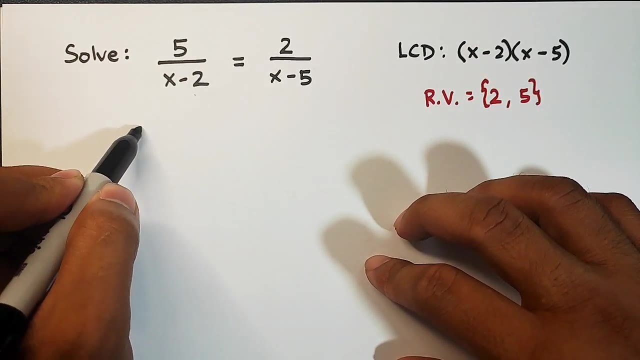 substitute positive 5, it will become 5 minus 5 and it will become undefined. Okay, let's continue. Since we already identified the LCD, or the least common denominator of this equation, we will multiply the whole equation using this, So it will go like this: 5 over. 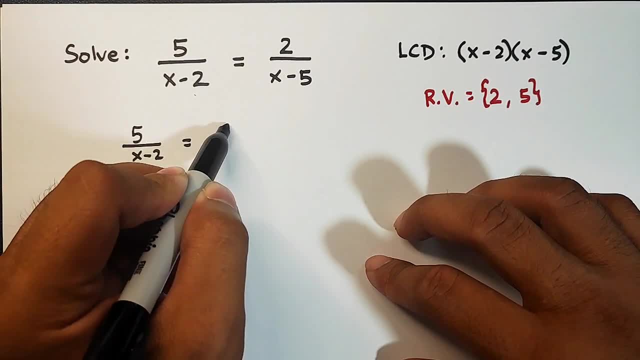 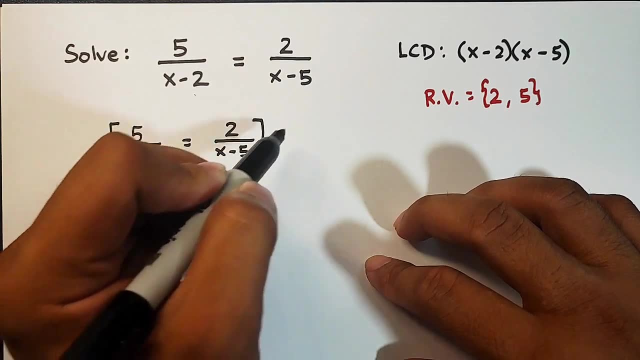 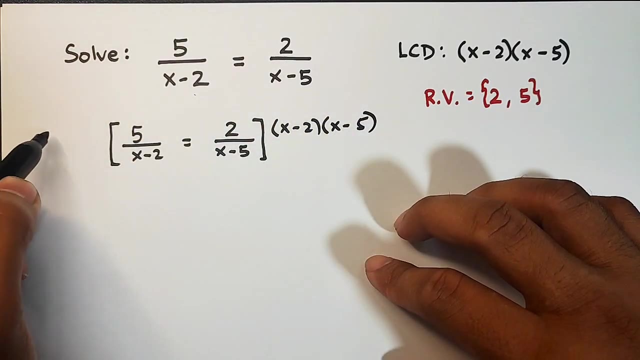 x minus 2 is equal to 2 over x minus 5.. Let's multiply them. Here: x minus 2 times x minus 5.. Here, on the other side, x minus 2 times x minus 5.. So, when we multiply them, what will happen is that you will distribute this one by one. 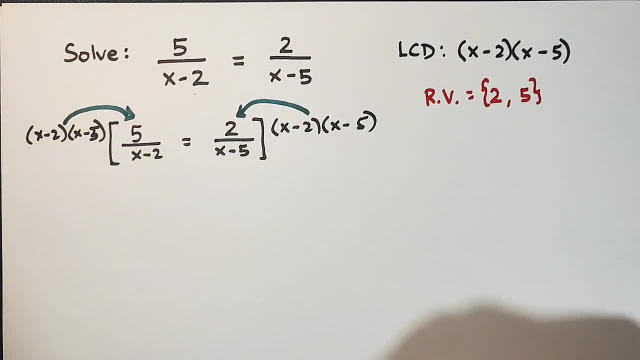 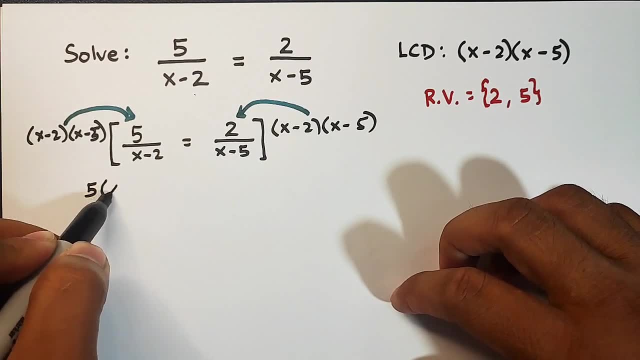 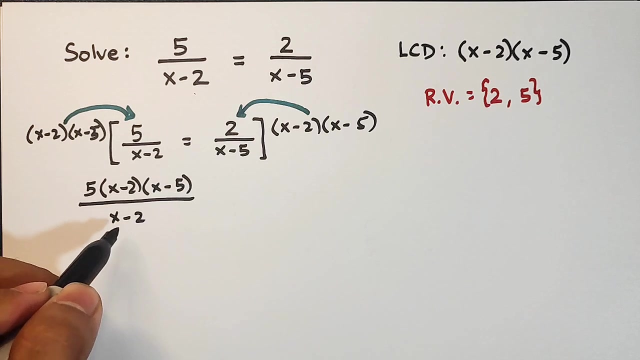 here and here and it will become like this: We have 5 times. we will put this one here and it will become x minus 2 times x minus 5, and then copy your denominator. By the way, guys, our main purpose. why do we need to do it this way? Because we need to eliminate. 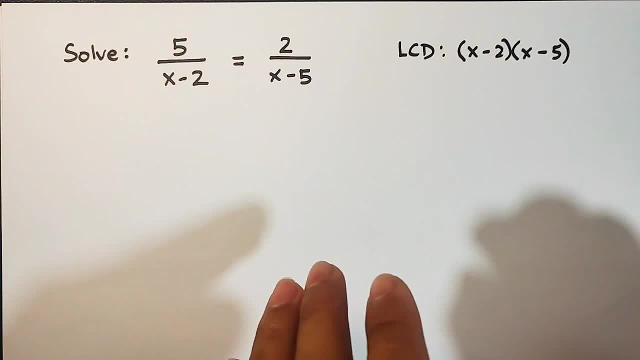 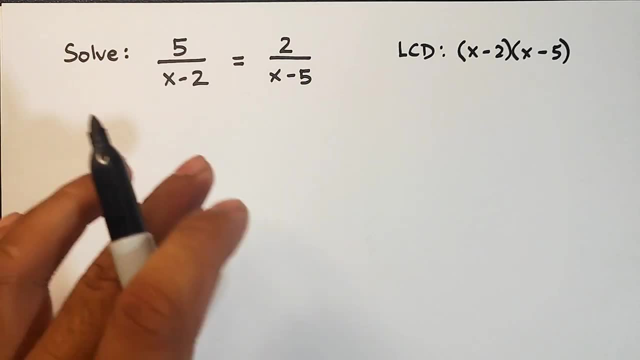 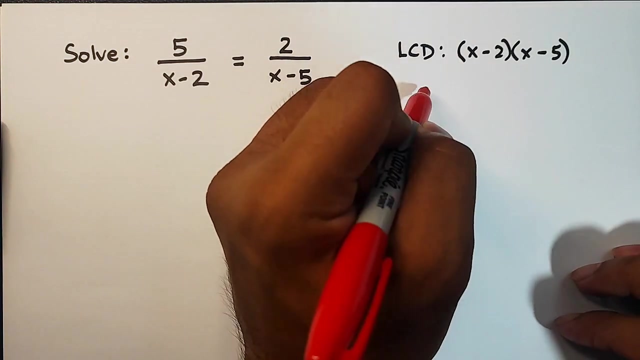 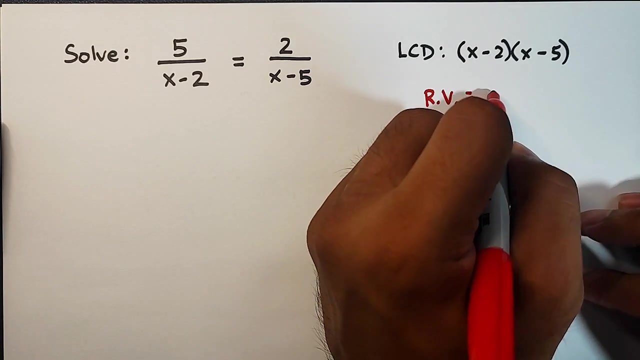 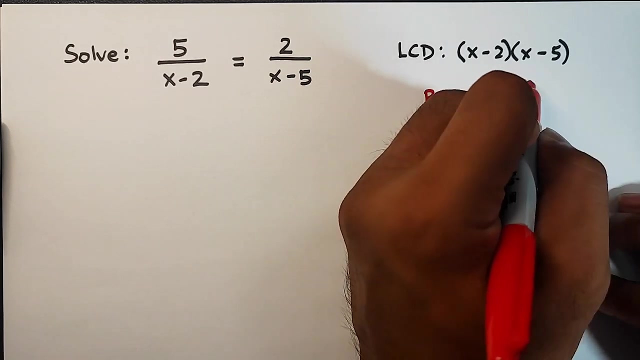 need to multiply it. So it is x minus 2 times x minus 5.. And, by the way, guys, before we proceed in solving this equation, let's identify our restricted value. Our restricted value, or RV, is positive 2 and positive 5.. So why is the restricted value 2 and positive 5?? 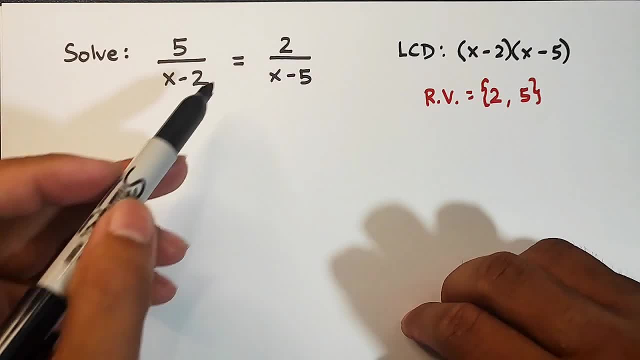 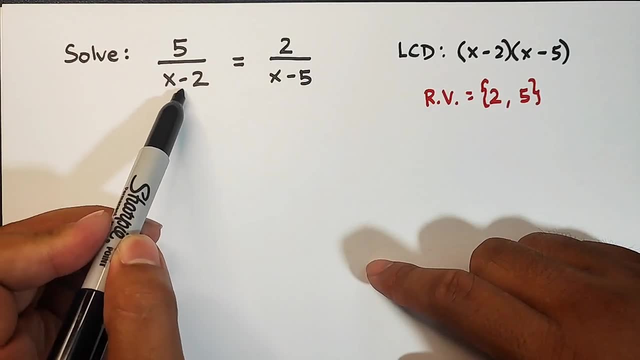 What this means is that they cannot be the value of x, because it will cause your denominator to be equal to 0. Imagine when you substitute the value of x as 2, that is, 2 minus 0, it will become undefined. 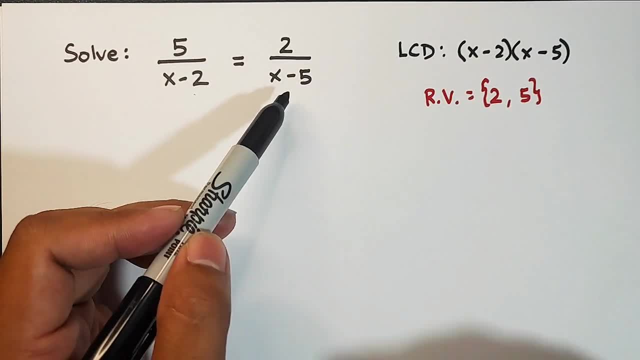 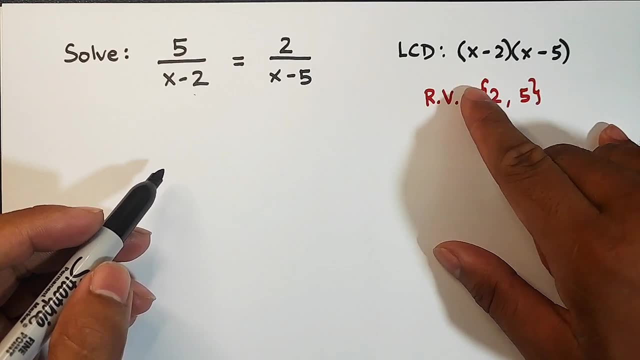 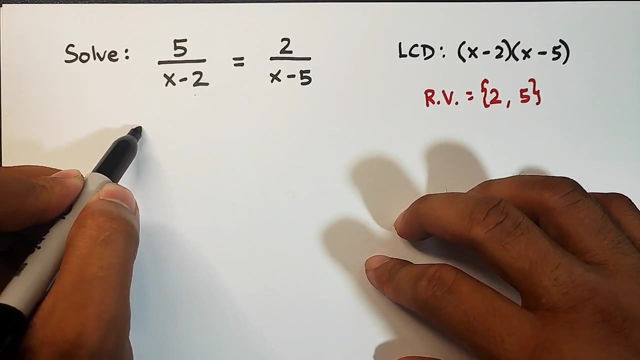 It will become 5 minus 5 and it will become undefined. Okay, let's continue. Since we already identified the LCD or the least common denominator of this equation, we will multiply the whole equation using this. So it will go like this: 5 over x minus 2 is equal to. 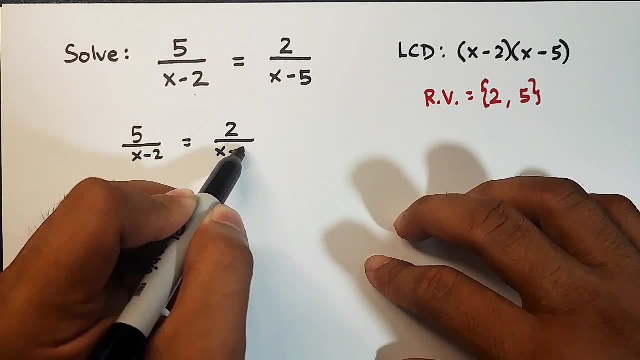 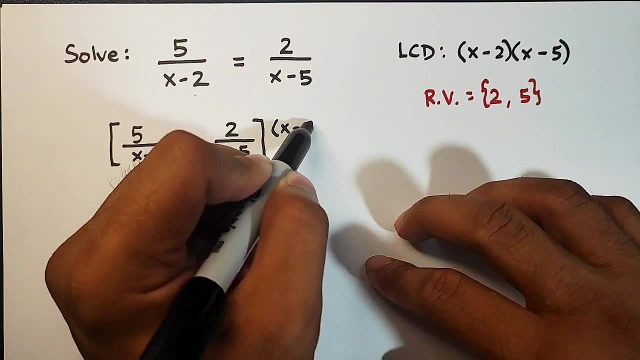 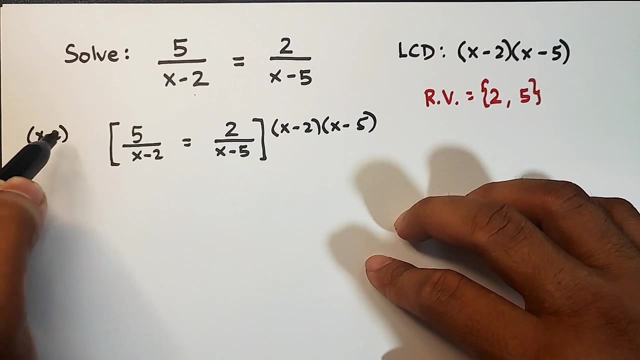 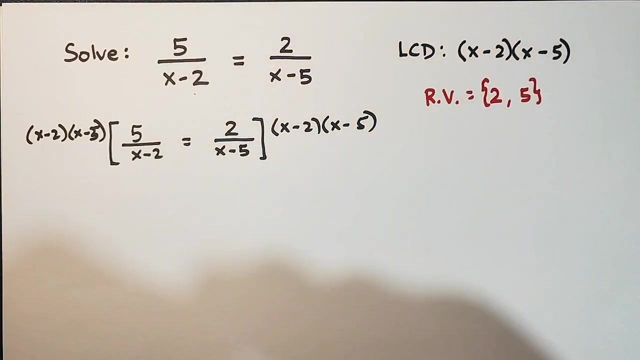 2 over x minus 5.. Let's multiply them Here: x minus 2 times x minus 5.. Here on the other side, x minus 2, x minus 5.. So when we multiply them, what will happen is that you will distribute this one by one here and 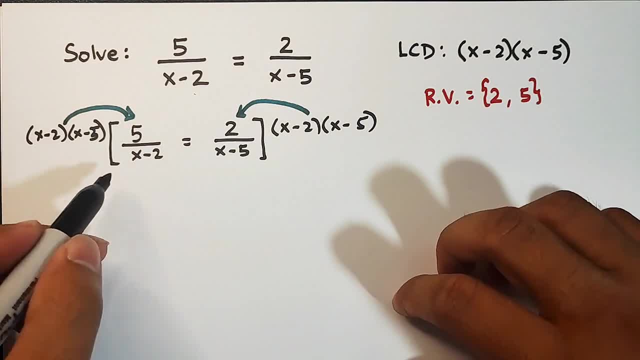 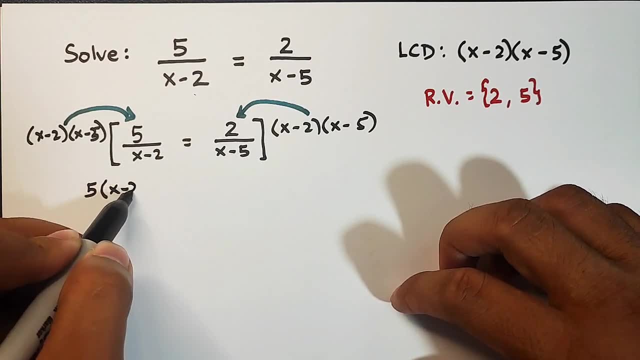 here and it will become like this: We have 5 times. we will put this one, We will put this one here: x minus 2 times, x minus 5, and then copy your denominator. By the way, guys, our main purpose. why do we need to do it this way? Because we need to eliminate your. 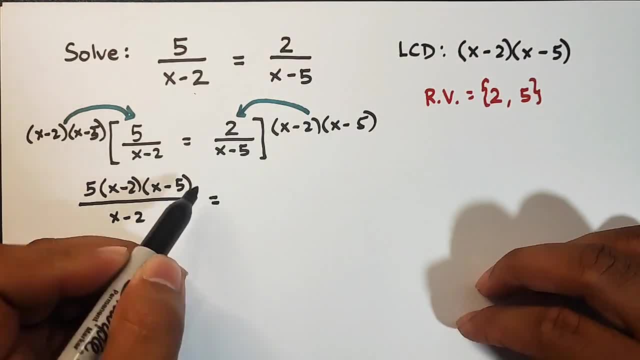 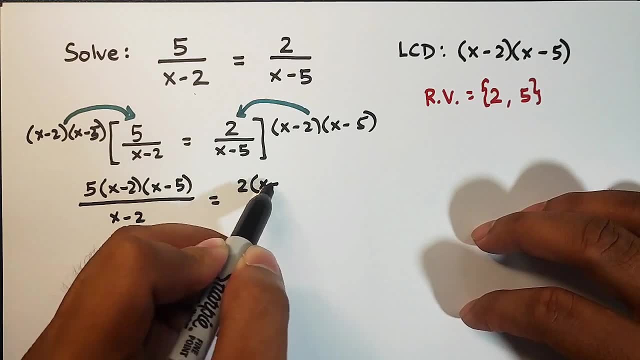 denominator, And later on you will see how- Then equal to 2 times x minus, 2 times x minus 5.. It will go like this: 2 times x minus 2, and then x minus 5 over x minus 5.. So we 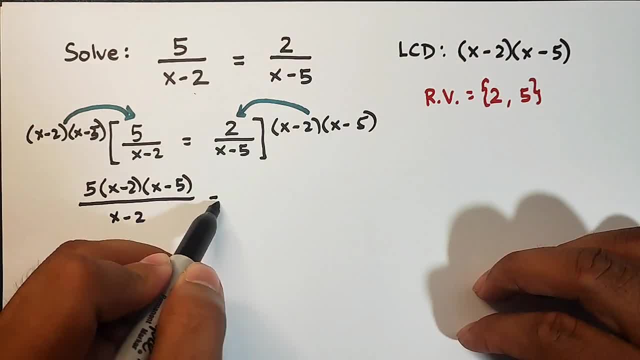 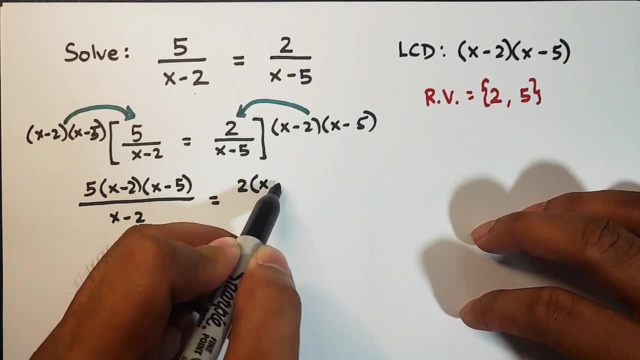 your denominator And later on you will see how. Then equal to 2 times x minus 2 times x minus 5.. It will go like this: 2 times x minus 2 and then x minus 5 over x minus 5.. 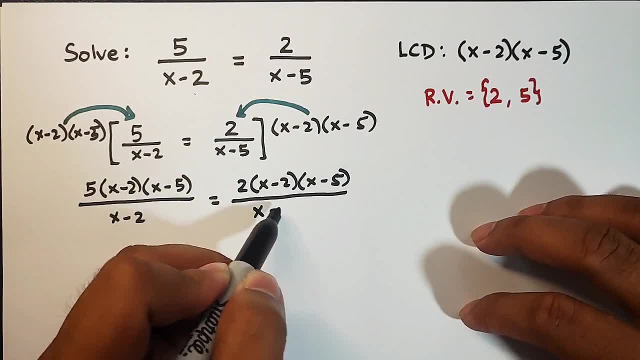 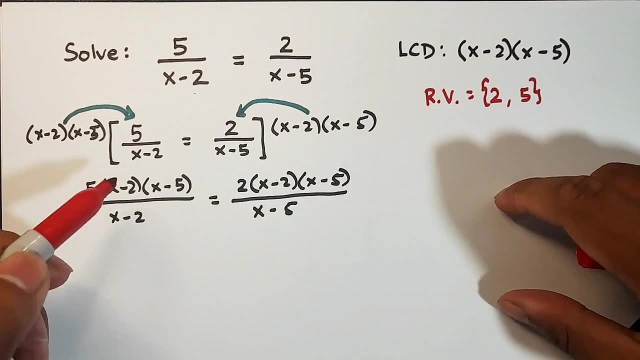 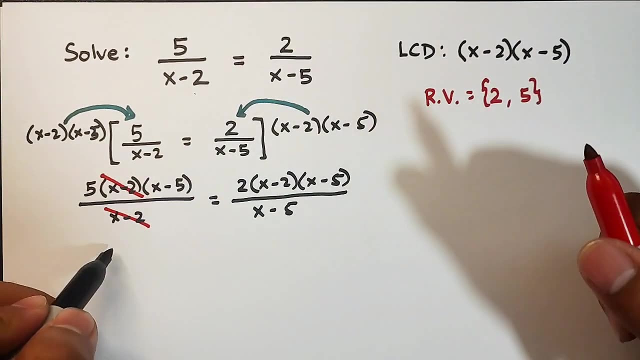 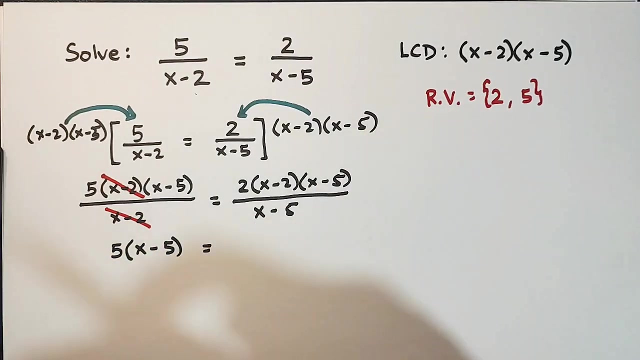 Copy your denominator. Copy your denominator: x minus 5.. So, as you can see, we have common binomial here. We can cancel out this x minus 2, as well as this x minus 2.. So what will remain is that we have 5 times x minus 5 is equal to here, on the other side of the equation. 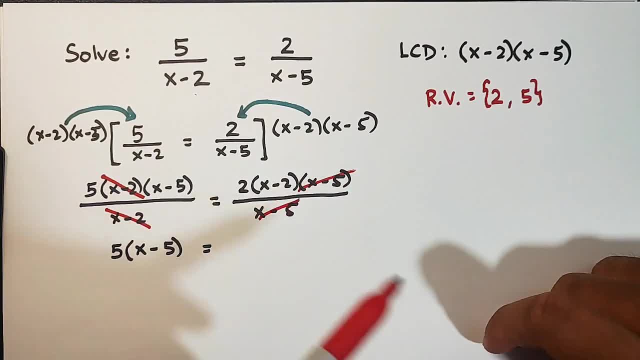 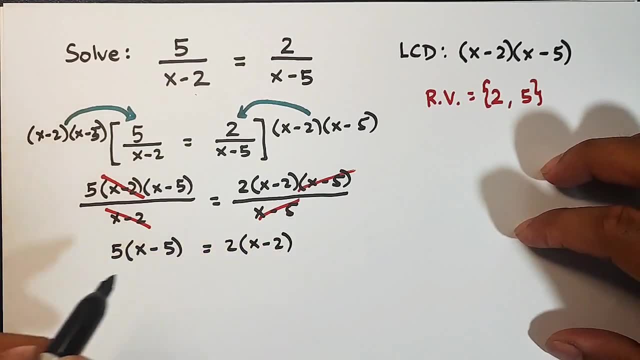 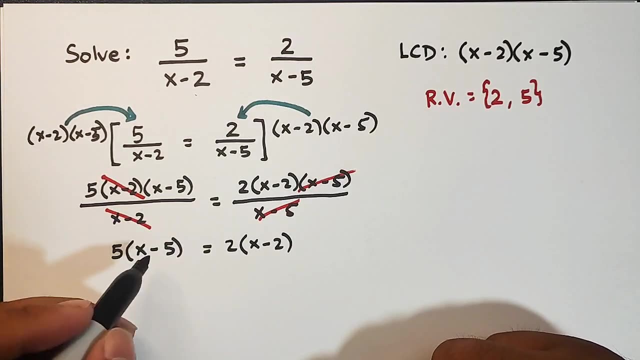 as you can see, we have similar x minus 5.. Cancel, cancel. So what we have here on the other side is 2 times x minus 2.. So remember yung parenthesis natin. it implies multiplication. Here we can use distributive property. 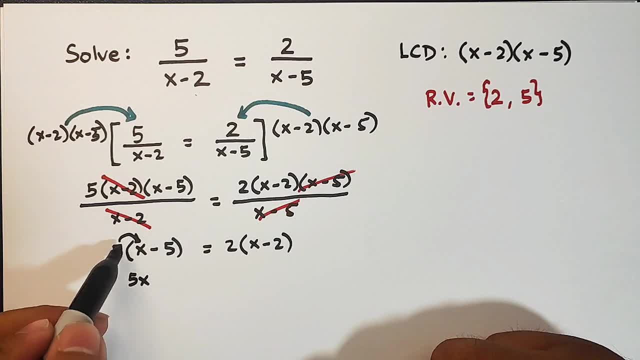 5 times x is 5x. 5 times negative, 5 is negative 25.. 5 here equal 2 times x, that is equal to 2x. then 2 times negative 2,, that is minus 4.. 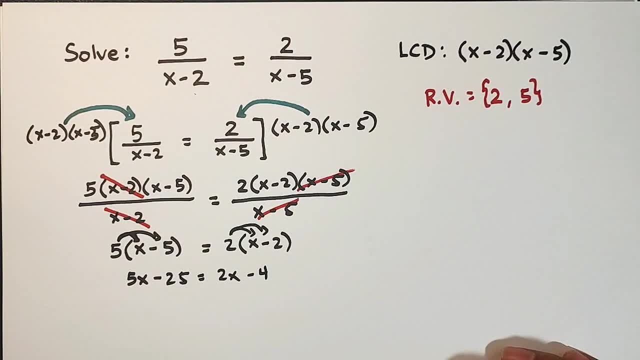 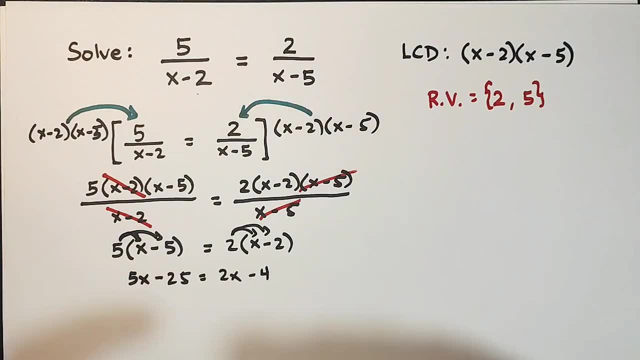 And what's next? We will combine like terms. So to combine like terms, guys, what we need to do is we will transpose 2x to the other side. So let's use different ink here, okay, and combine with 5x. 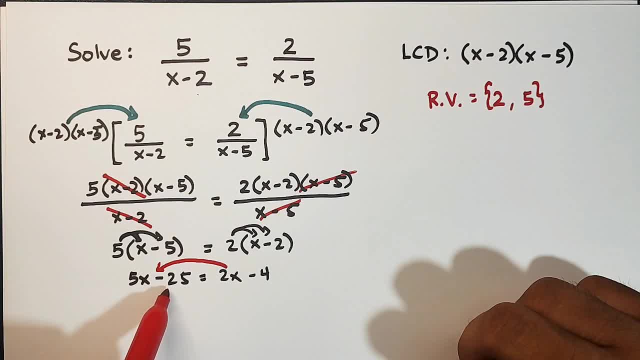 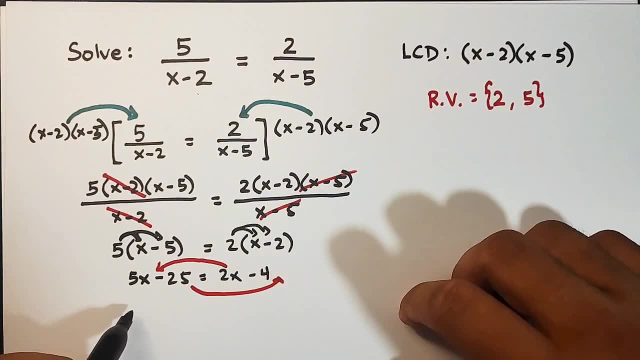 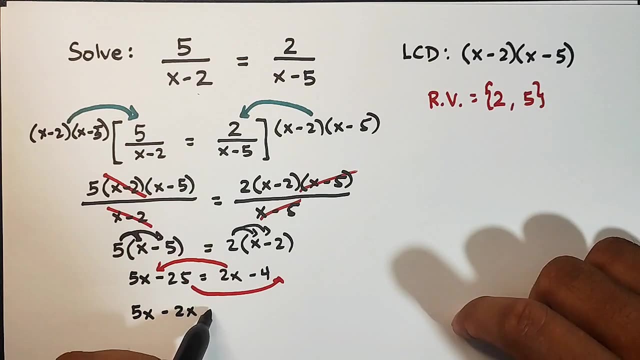 And we will also transpose So 20, negative 25 to the other side. combine it with negative 4.. So what will happen is that we will copy 5x and this 2x will become negative. 2x is equal to negative 4 plus 25.. 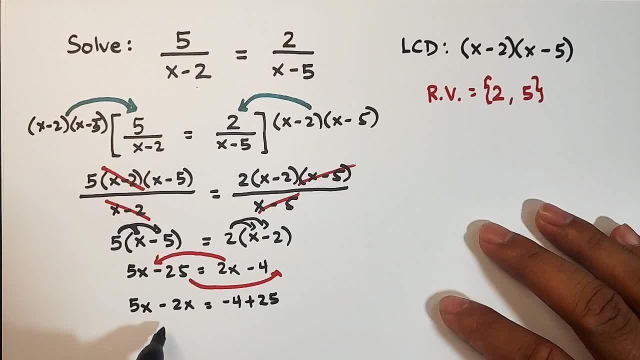 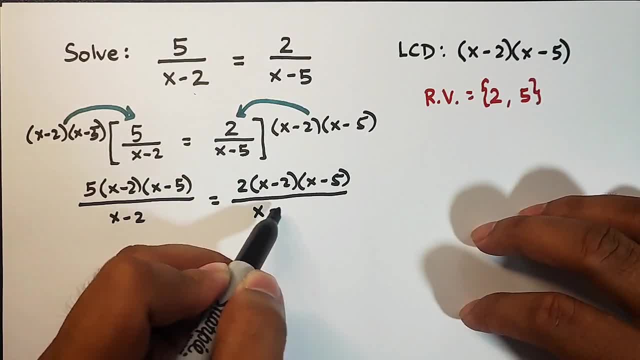 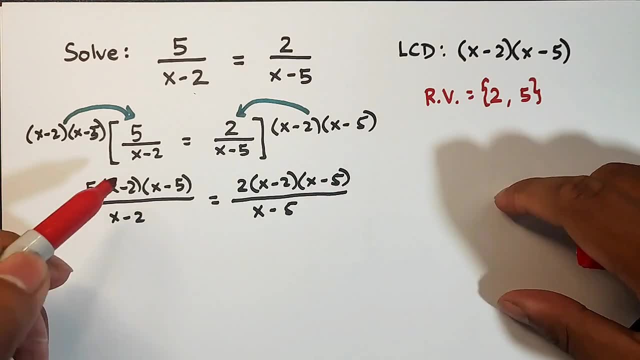 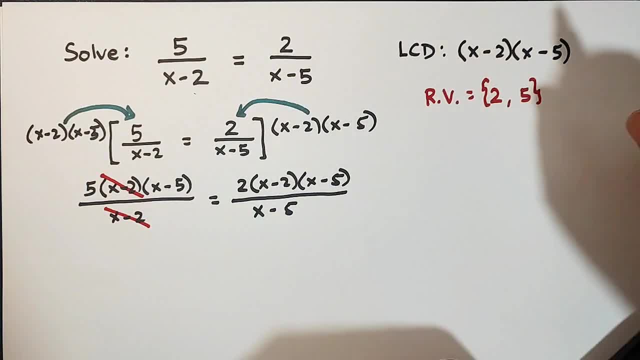 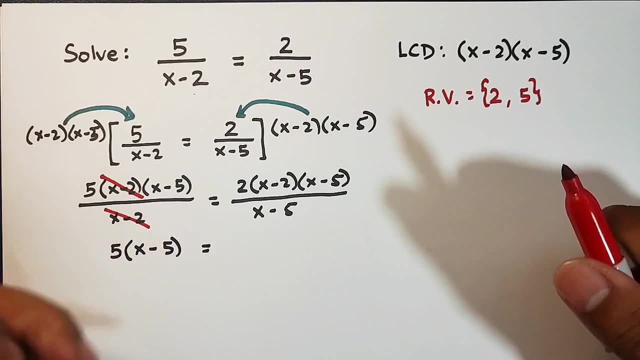 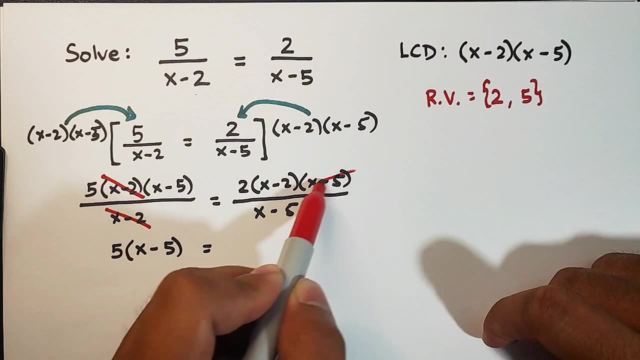 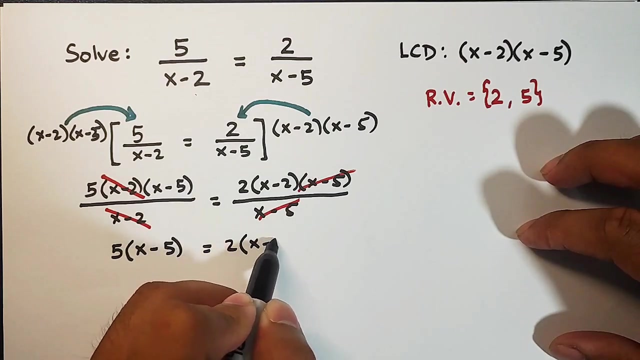 well as this, x minus 2.. So what will remain is that we have: 5 times x minus 5 is equal to. here on the other side of the equation, as you can see, we have similar x minus 5 here: Cancel, cancel. So what we have here on the other side is 2 times x minus 2.. So 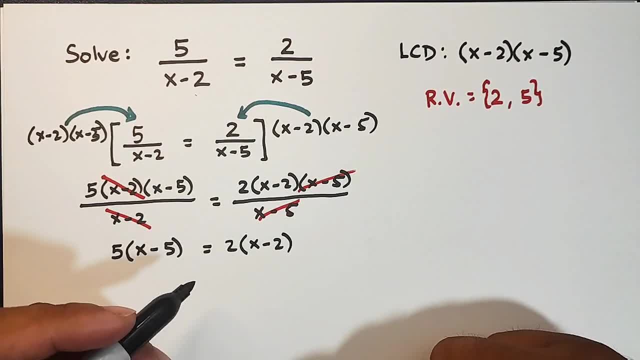 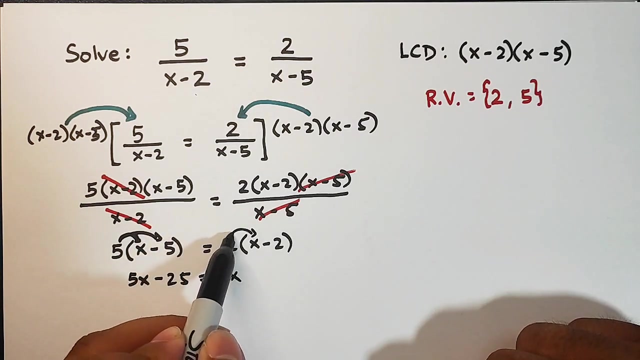 remember yung parenthesis natin. it implies multiplication. Here we can use distributive property: 5 times x is 5x. 5 times negative, 5 is negative 25.. Here, equal 2 times x, that is equal to 2x. Then 2 times negative, 2, that is minus 4.. And what's next? We will. 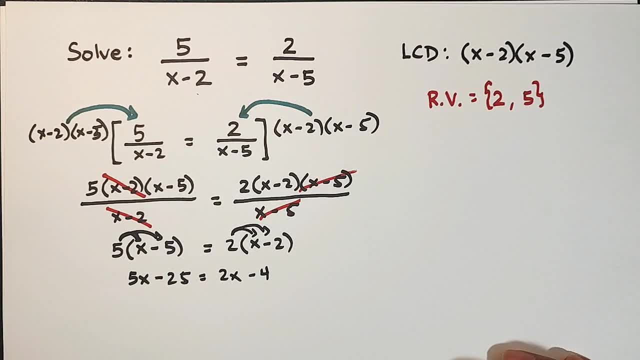 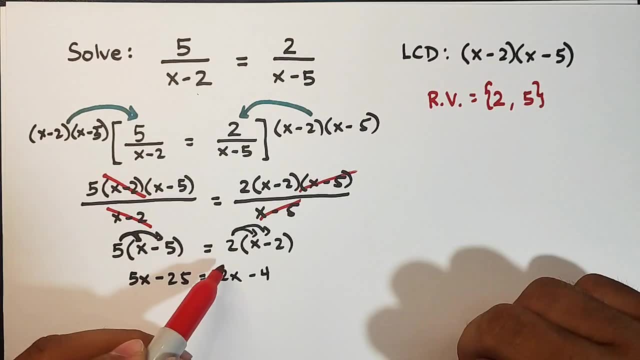 combine like terms. So, to combine like terms, guys, what we need to do is we will transpose 2x to the other side- So let's use different ink here, Okay- And to combine with 5x, And we will also transpose negative 25 to the other side. 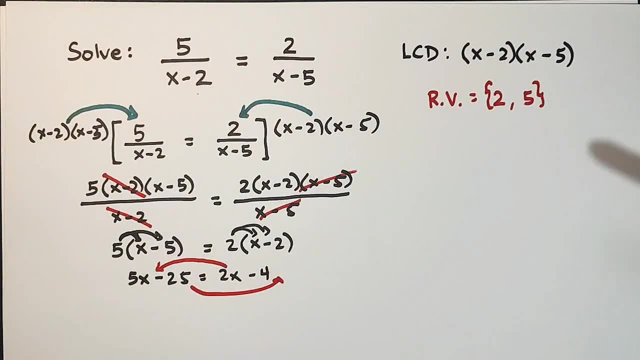 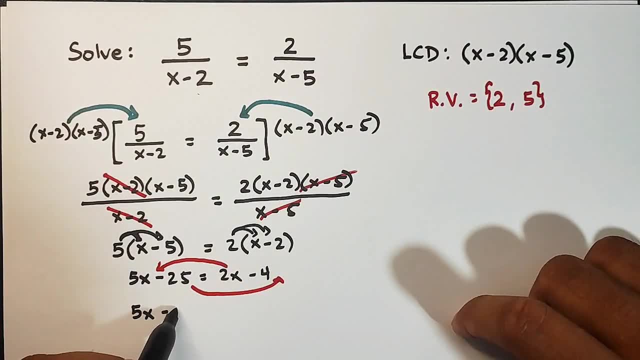 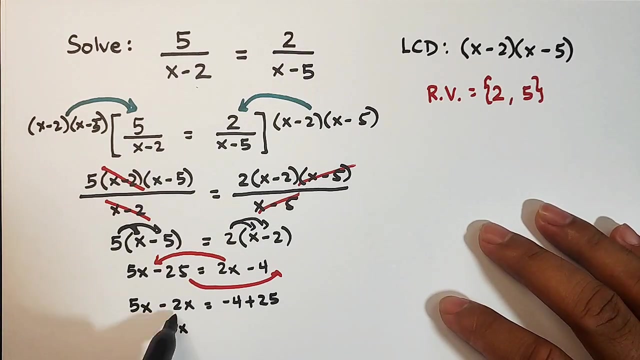 Combine it with negative 4.. So what will happen is that we will copy 5x And this 2x will become negative. 2x is equal to negative, 4 plus 25.. And, simplifying this equation, this will become 3x. 5x minus 2x is 3x is equal to 21.. 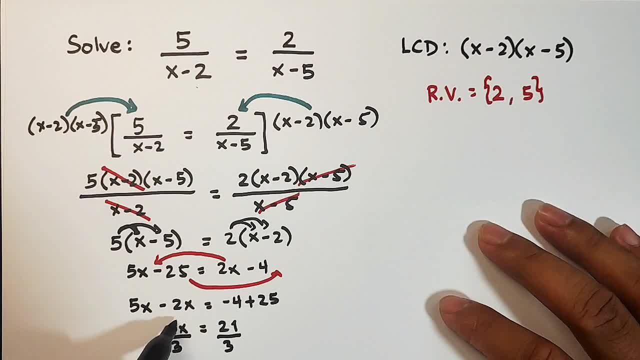 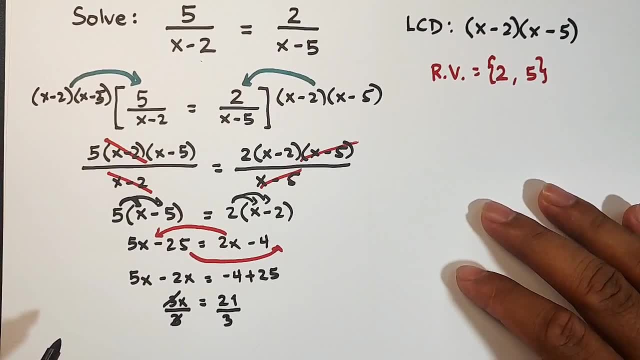 Divide both sides by 3.. Divide both sides by 3.. Cancel. cancel Your x. okay, we will adjust this one. Your x now is equal to 7.. This is now the answer. Or lagay natin dito. 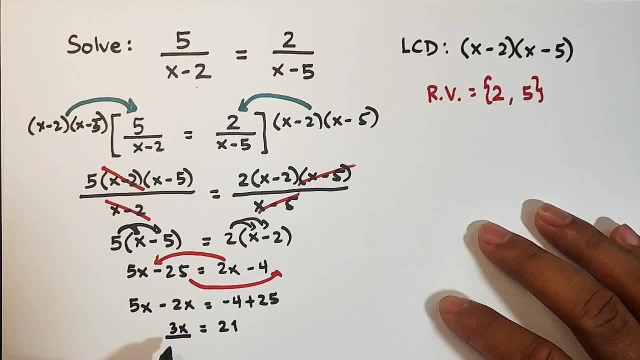 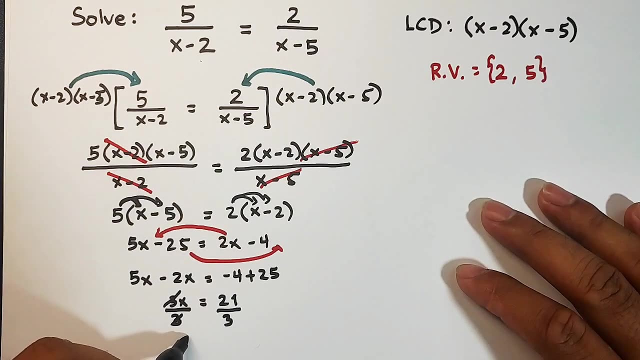 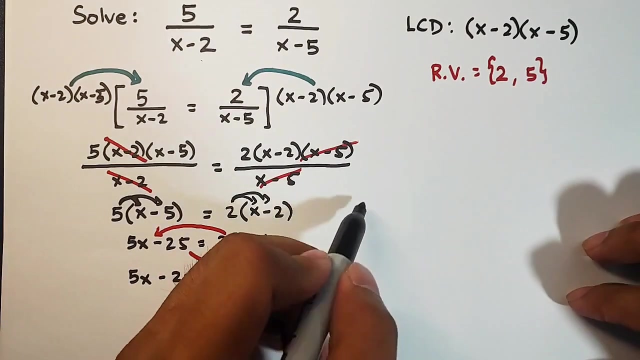 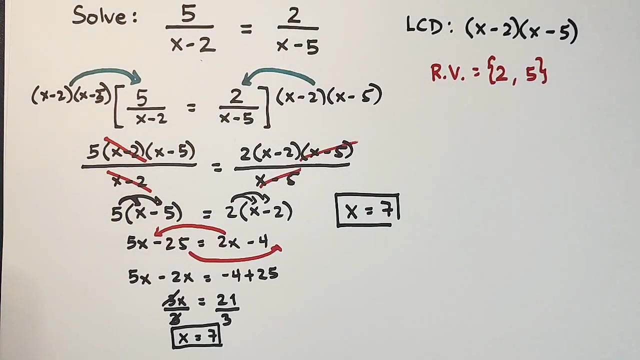 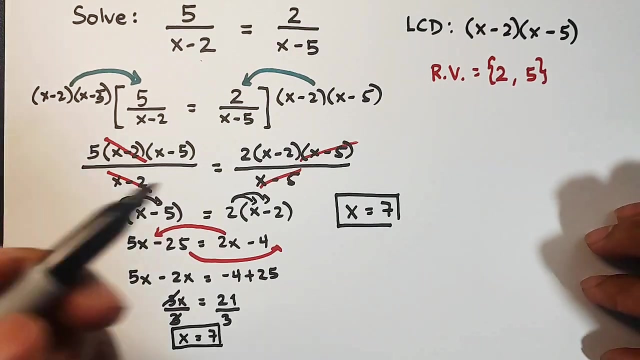 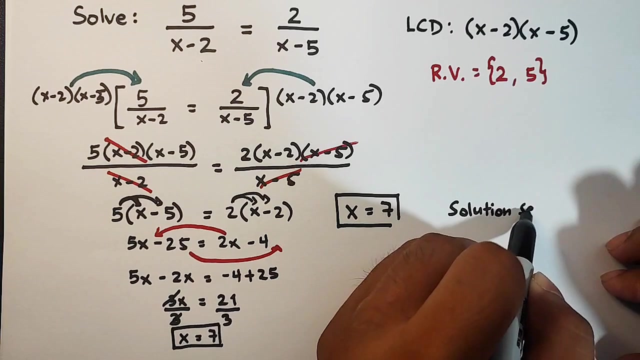 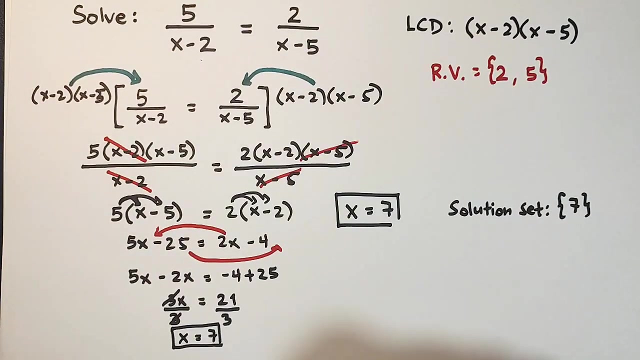 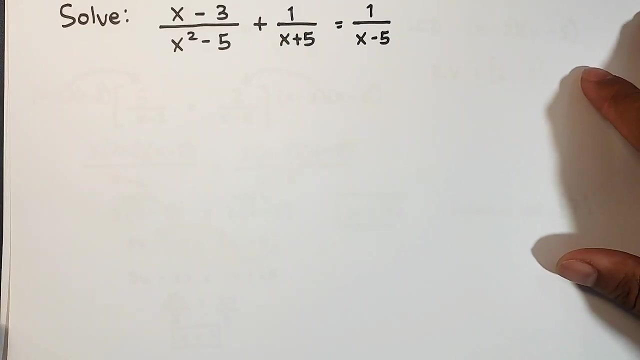 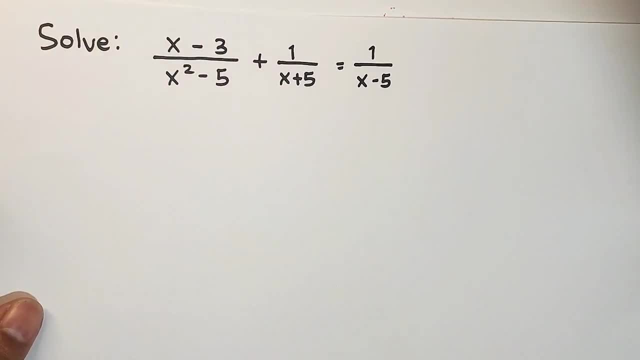 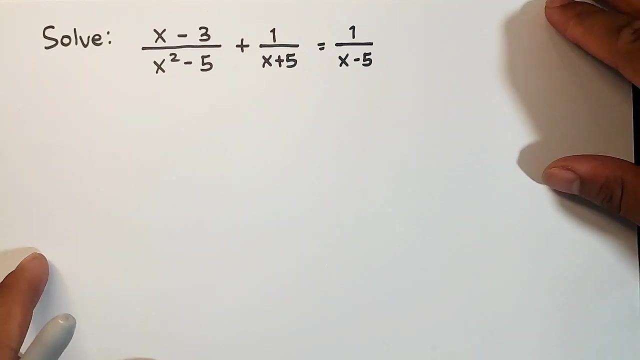 so let me remove the other problem. so we have here x minus 3 over x. squared minus 5 plus 1 over x plus 5 is equal to 1 over x minus 5. now he thinks the problem is hard. don't worry guys. 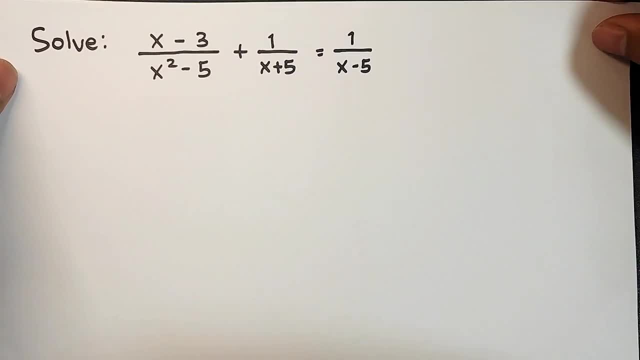 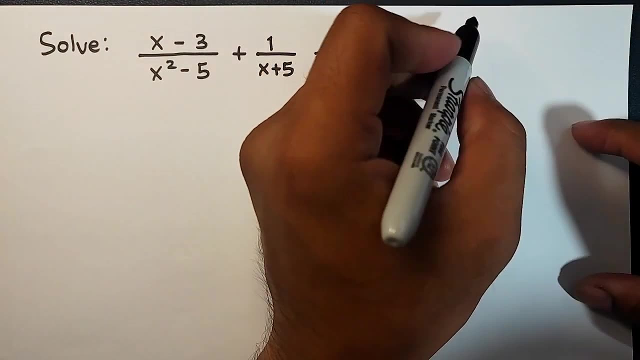 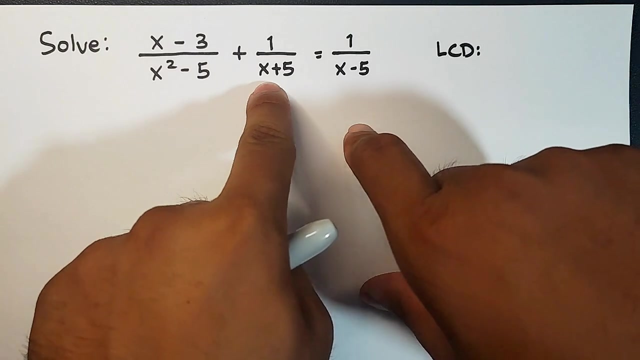 because in this problem- let me show you this problem properly- as you can see- to determine the LCD, LCD, tayo LCD. as you can see, we have here two different binomials: x plus 5 and x minus 5, so we also have x squared minus 5. 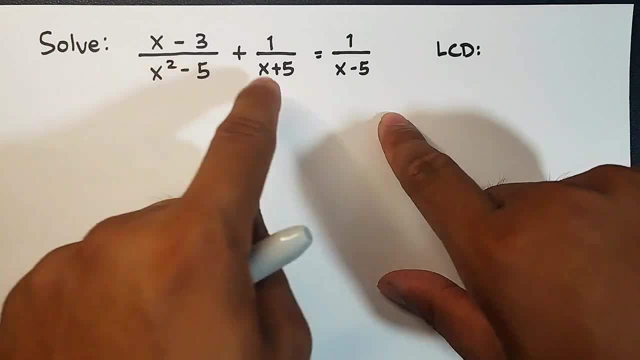 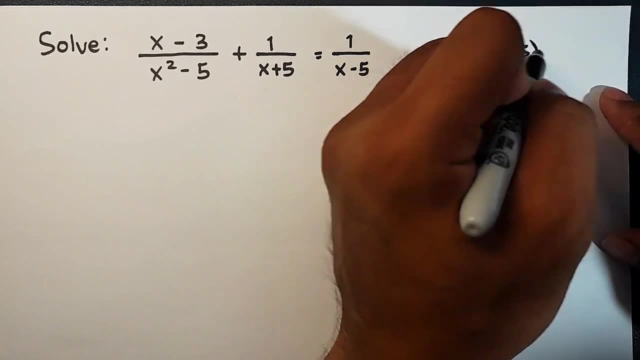 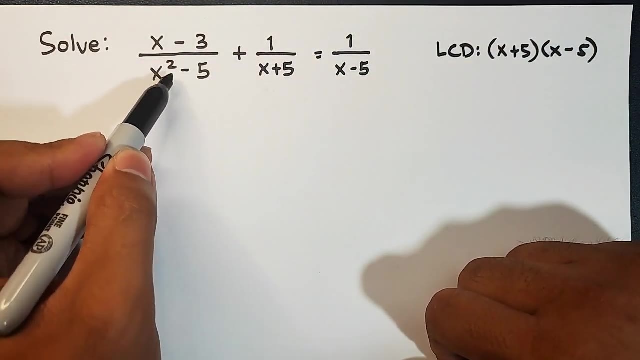 the factors of x squared minus 5 are this: x plus 5 times x minus 5, meaning the LCD is simply x plus 5 times x minus 5. that's it, guys. now try to factor this out first, because what they are doing here to see the actual factor. 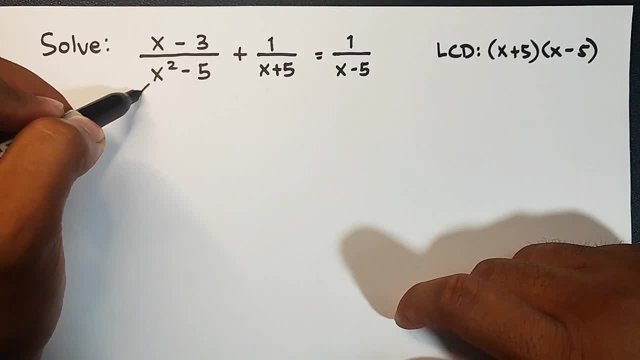 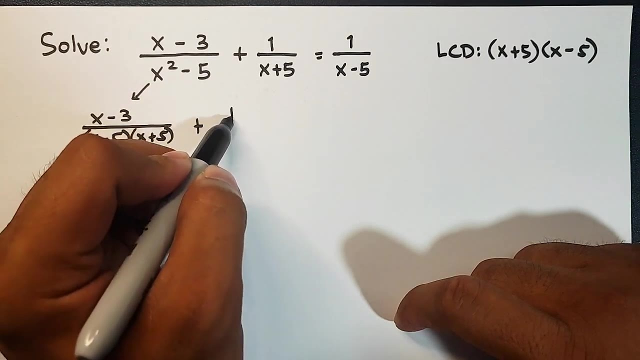 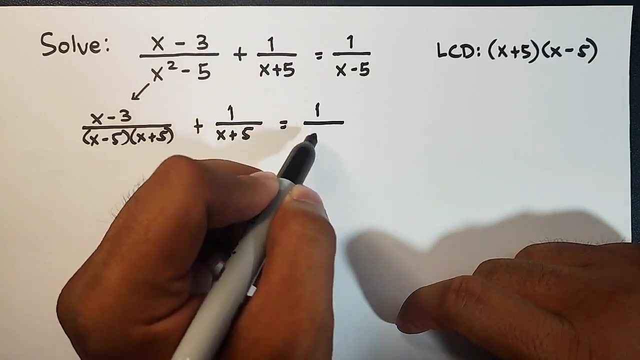 is they are factoring the denominator, so let's express it so it will become x minus 3 over x minus 5 over x squared minus 5 times x plus 5. then plus 1 over x plus 5 is equal to 1 over x minus 5. 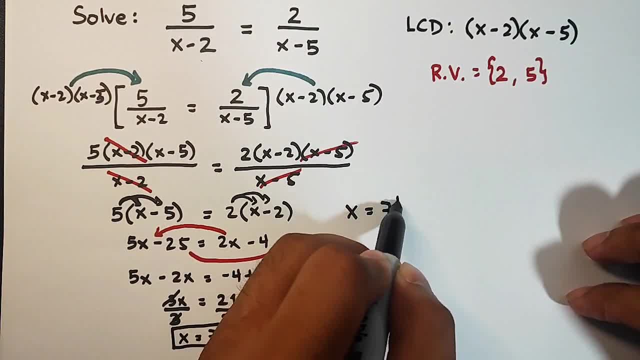 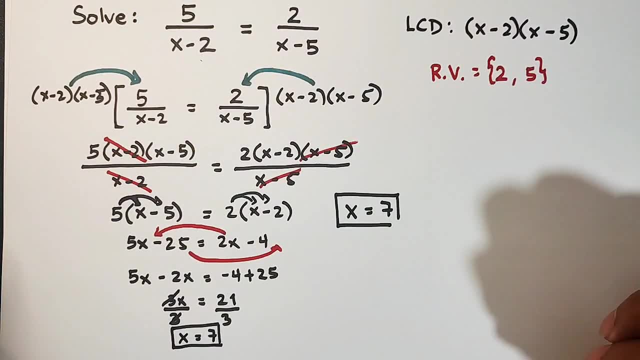 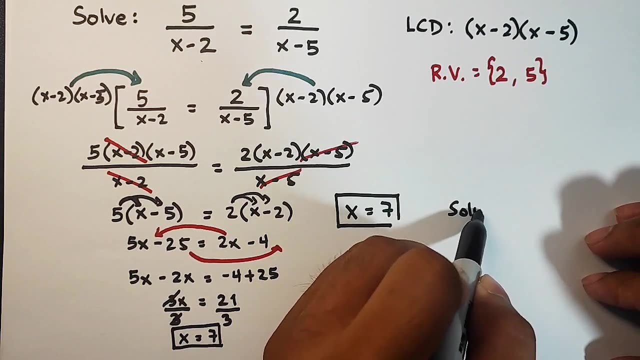 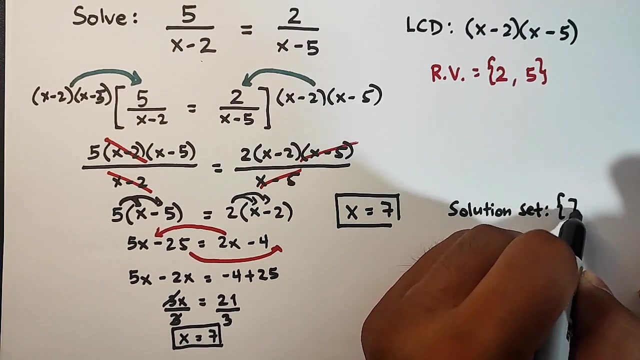 your x is equal to 7.. This is now the answer in this given, or the solution of this given rational equation. And if you want to express your, the value of x, in solution set, pwede mo siyang gawin ganito: solution set is this: 7.. Ganito siya yung sulat. Okay, Now let's. 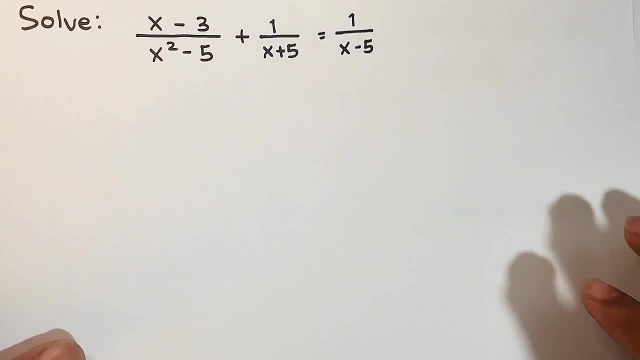 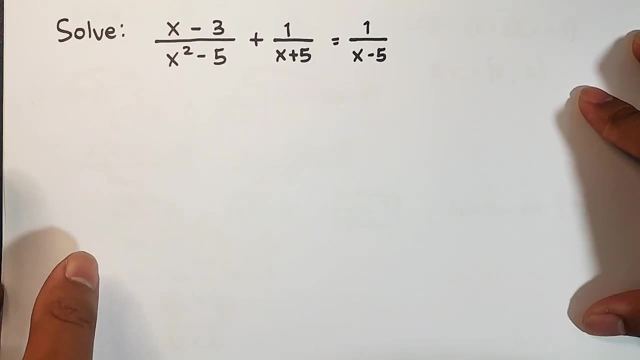 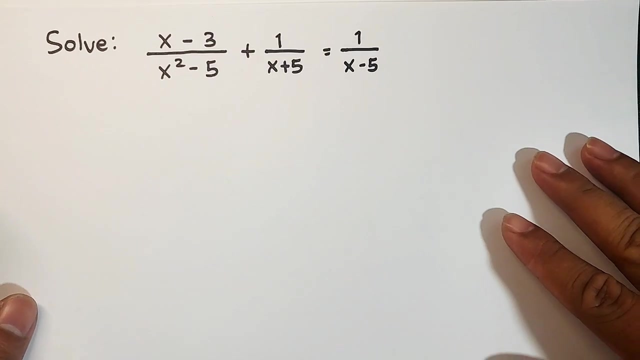 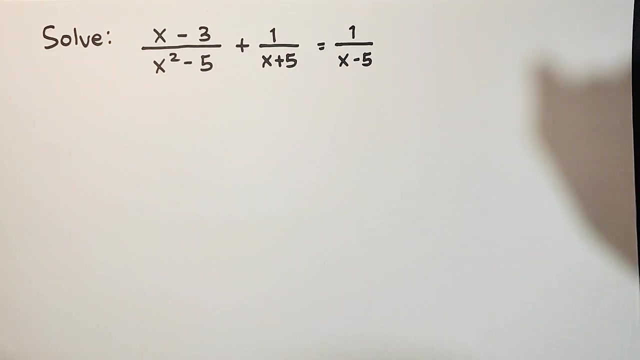 move on with another example. So what we have here, as you can see, is a little bit complicated type of problem. So let me remove the other problem. So we have here x minus 3 over x. squared minus 5 plus 1 over x plus 5 is equal to 1 over x minus 5.. Now isipin niya mahirap. 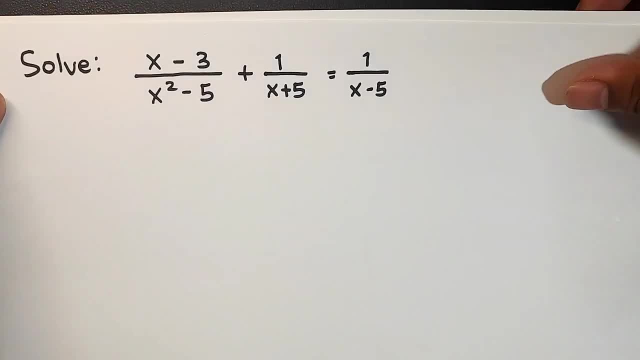 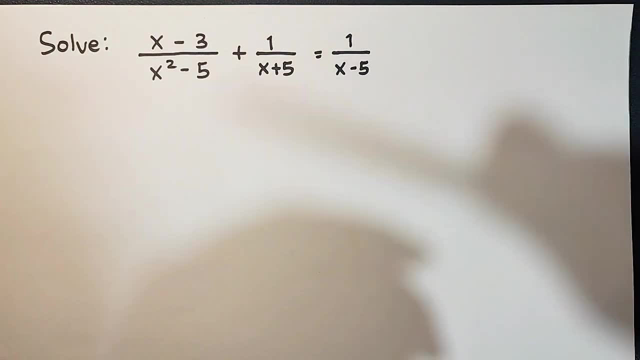 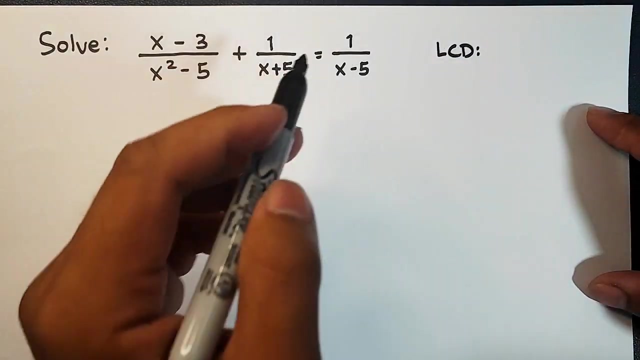 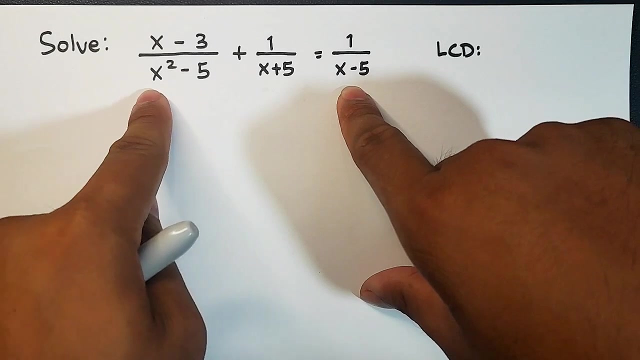 yung problem. Don't worry, guys, because in this problem- let me show you this problem- As you can see, to determine the LCD, LCD, tayo LCD. as you can see, we have here two different binomials: x plus 5 and x minus 5.. So we also have x squared minus 5.. The factors of x squared: 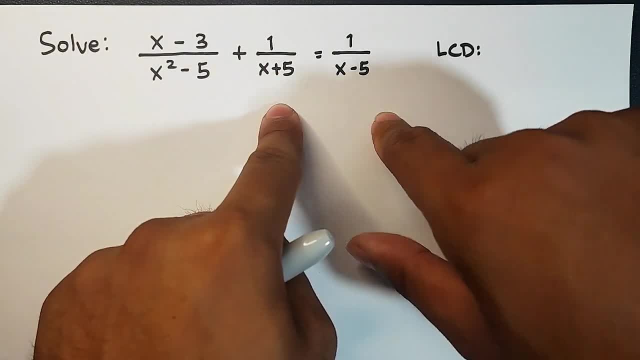 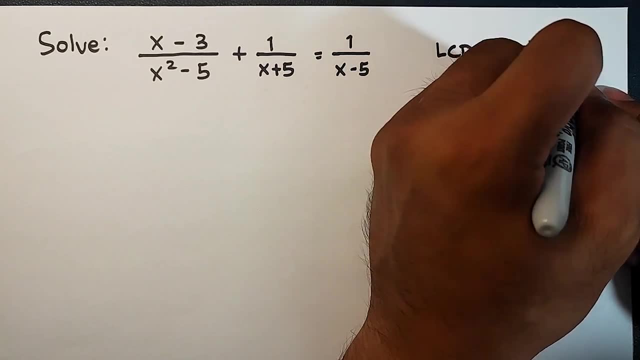 minus 5 are this x plus 5 times x minus 5, meaning the LCD is simply x plus 5, x plus 5 times x minus 5.. That's it, guys. Now try to factor this out first. kasi yung gina. 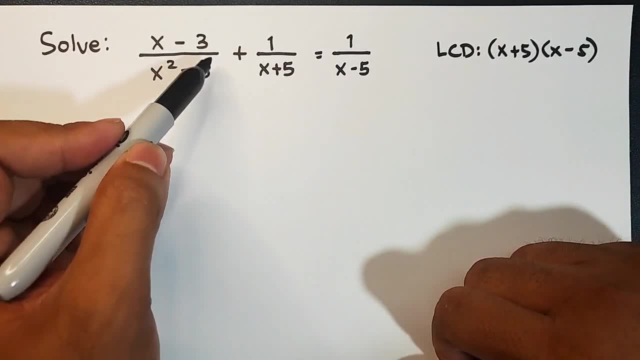 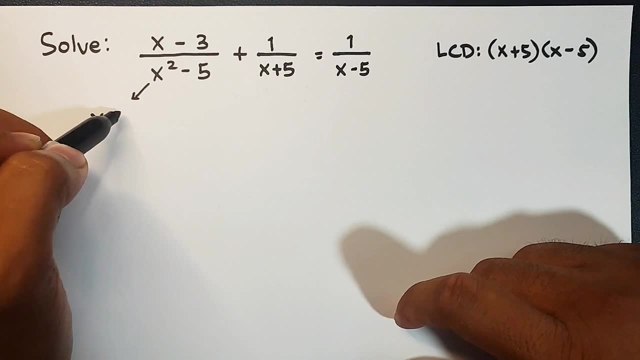 gawin dito para makita talaga yung tunay na factor is they are factoring the denominator, So express mo rin natin. So it will become x minus 3 over x minus 5 times x plus 5.. Then 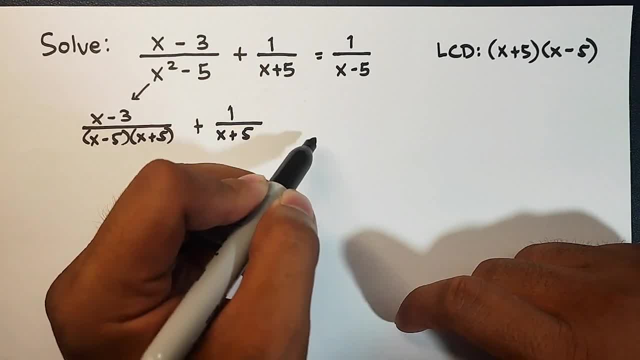 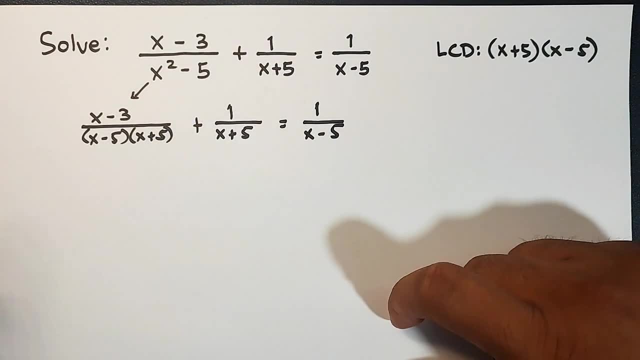 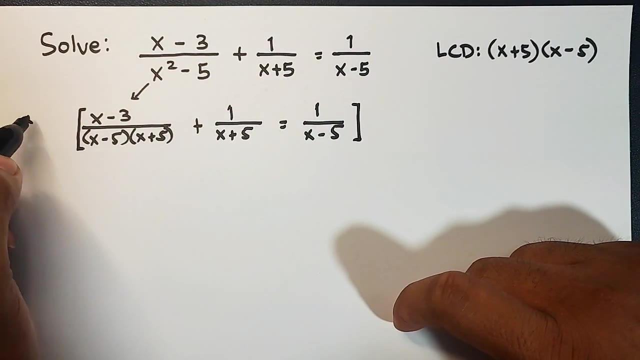 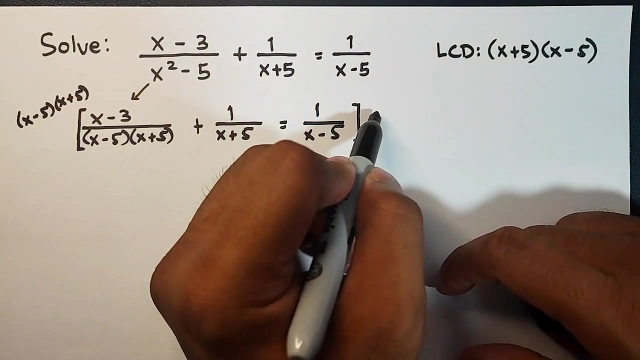 we will have: one over x plus 5 is equal to one over x minus 5.. In same process we will multiply the whole equation by the LCD. we have x minus 5 times x plus 5.. Here also x minus 5 times x plus 5.. 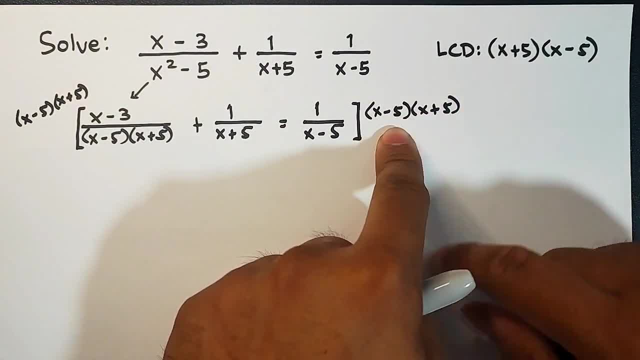 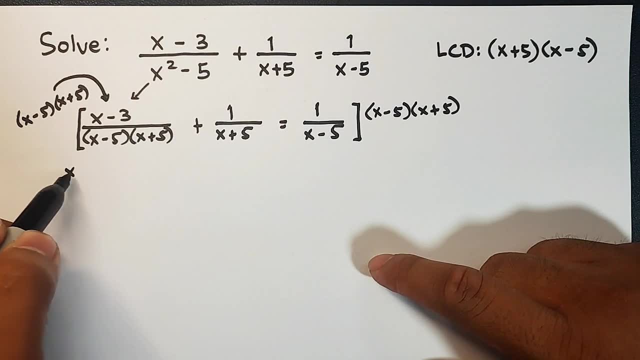 So pay attention, guys, I'm just going to give you a little development here. So if you They can interchange guys, You can change the position of this. So when multiplying guys, multiply it, It will become x minus 3. 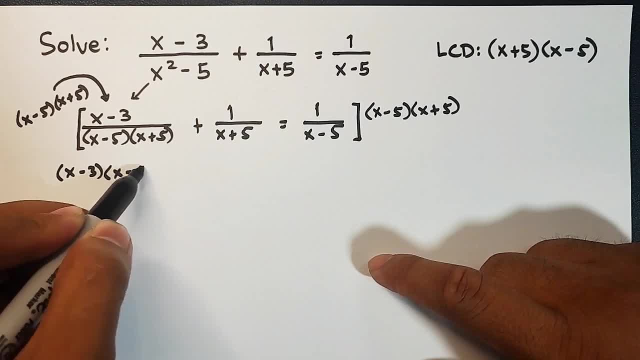 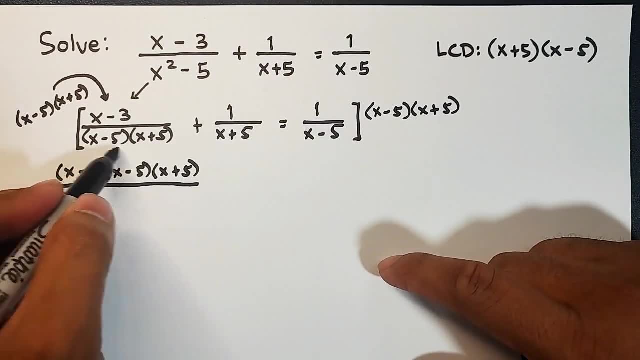 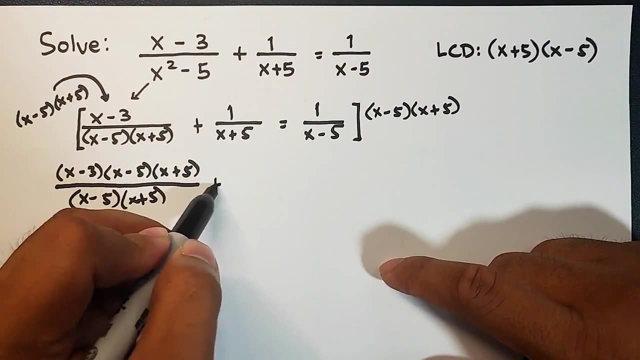 times x minus 5 times x plus 5.. Actually you can cancel this out, but I'm showing you the proper solution. Copy your denominator x minus 5 times x plus 5 here, plus multiply this here to become x minus 5. 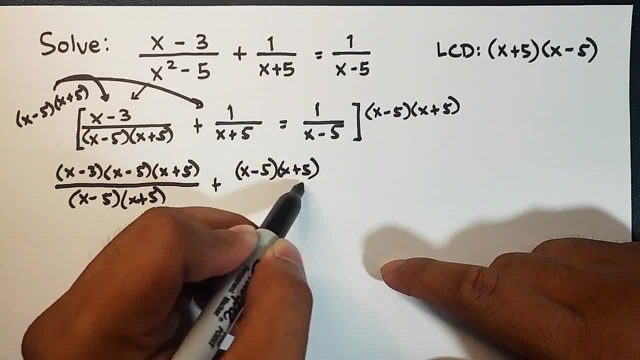 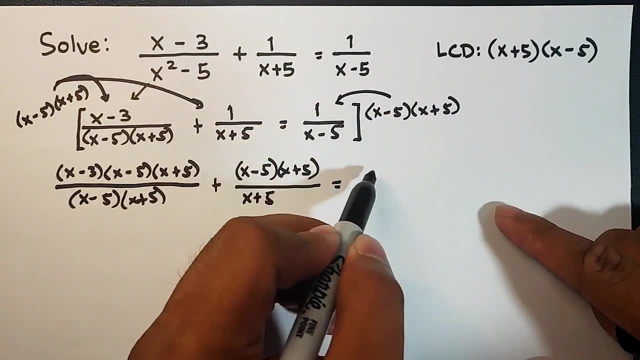 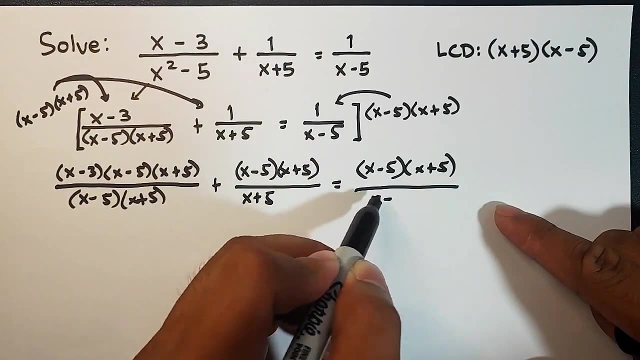 times x plus 5, because it's just 1 over x plus 5.. We just copied this. It's equal to multiply here. This is x minus 5 times x plus 5 over your denominator x minus 5.. As you can see, we can easily cancel out. 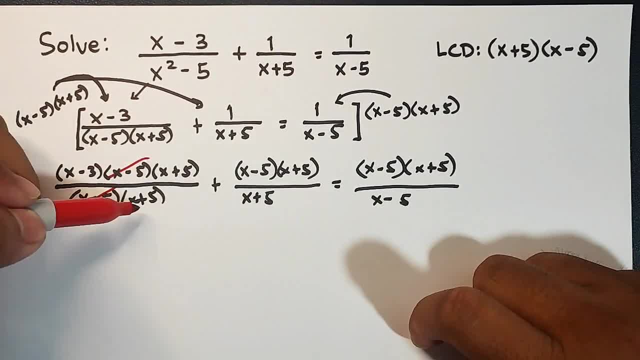 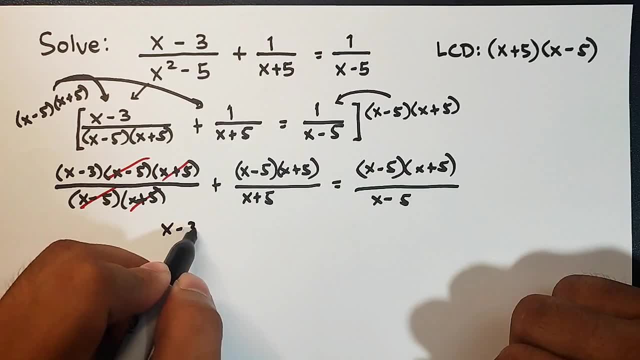 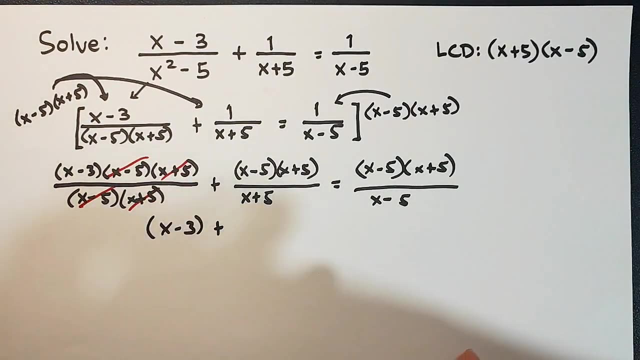 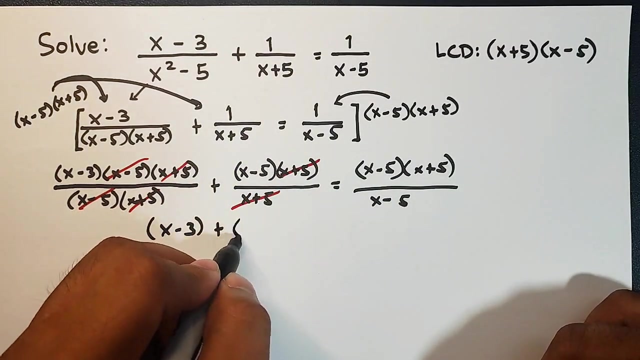 here: Common common, common, common. So what we have now is simply x minus 3. plus this, You can eliminate x plus 5 and x plus 5.. So what we have here is simply x minus 5.. 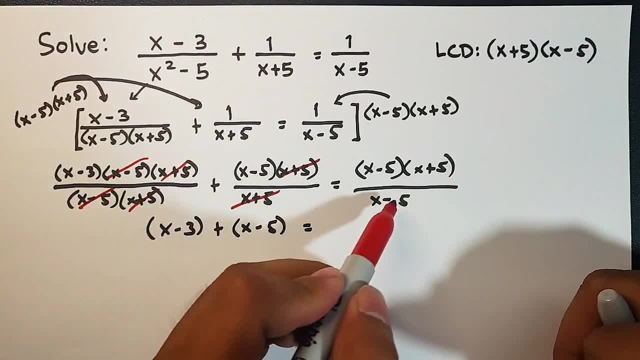 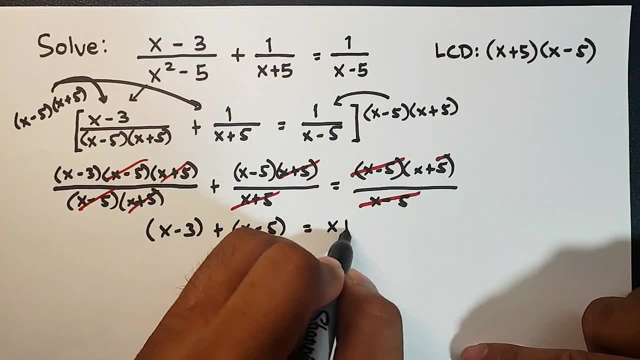 On the other side, we can cancel out x minus 5 and x minus 5.. So what will remain is x plus 5.. So, as you can see, it won't multiply because it has an addition. Let's just combine. 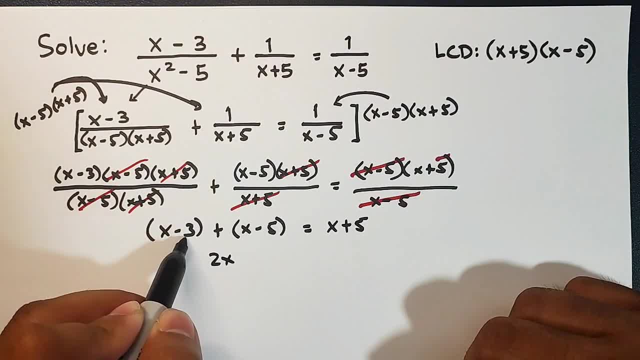 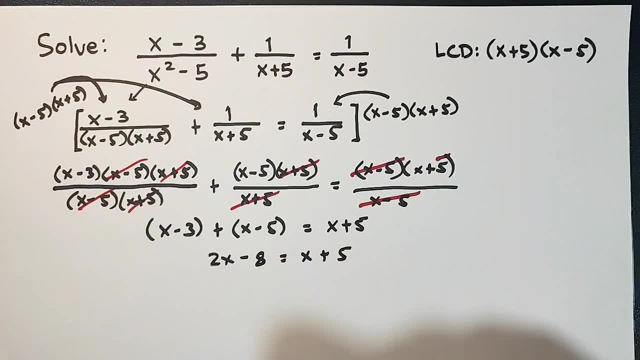 x plus x is 2x Negative. 3 plus negative, 5 is negative. 8 is equal to x plus 5.. Same scenario we will transpose again. we will transpose terms here and here. So we have 2x. 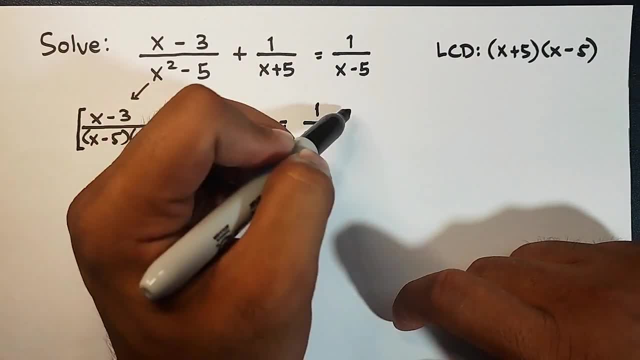 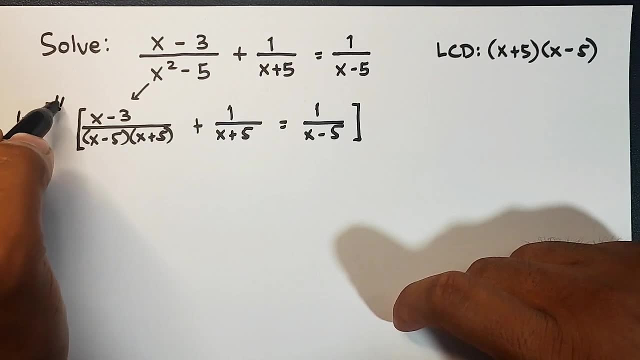 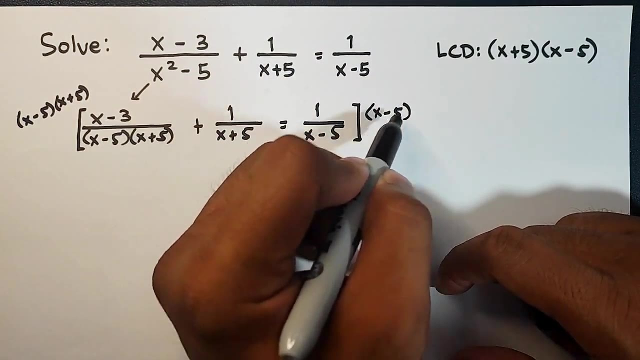 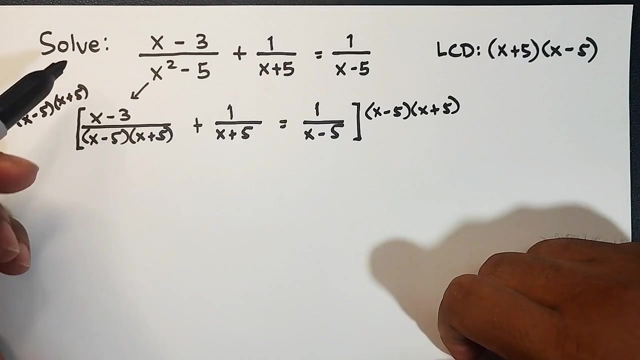 in the same process we will multiply the whole equation by the LCD. we have x minus 5 times x minus 5, x plus 5. here also x minus 5 times x plus 5, so they can interchange, they can change the position. so when multiplying, 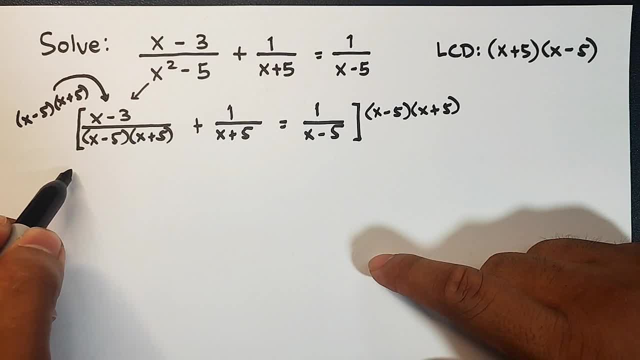 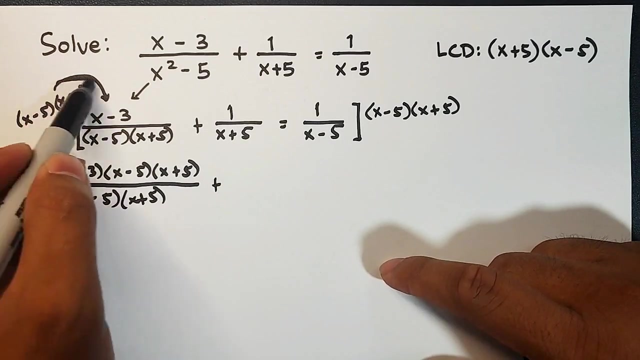 let's multiply, it will become x minus 3 times x minus 5 times x plus 5. actually, you can cancel this out, but I am showing you the proper solution. copy your denominator x minus 5 times x plus 5 here, plus multiply this here. 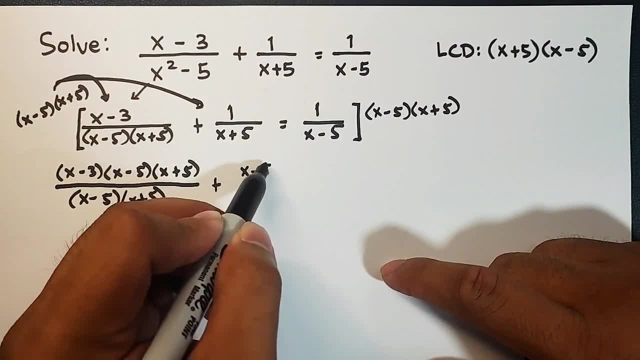 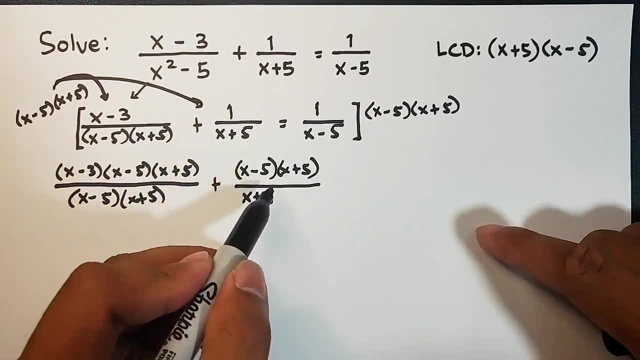 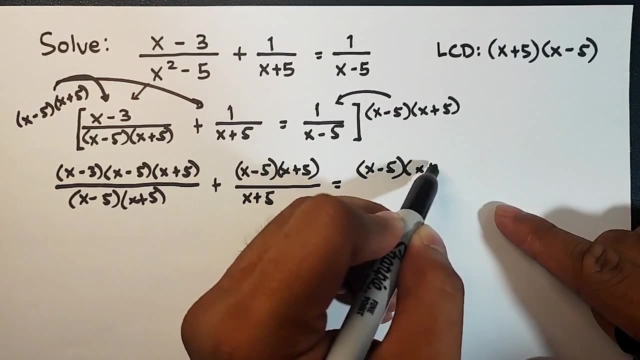 to become x minus 5 times x plus 5, because it's just 1 over x plus 5. we just copied this is equal to multiply here. this is x minus 5 times x plus 5 over your denominator x minus 5. as you can see, 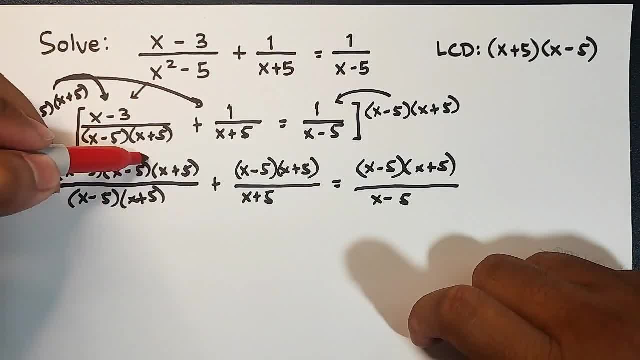 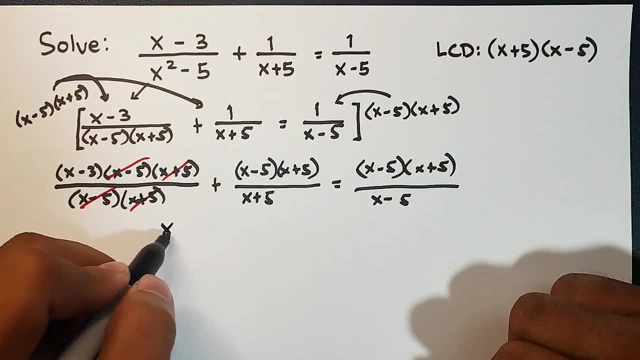 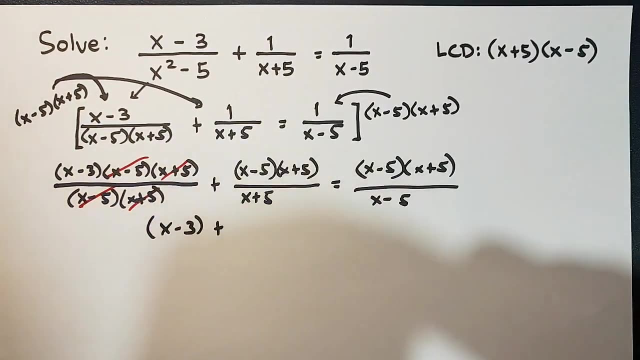 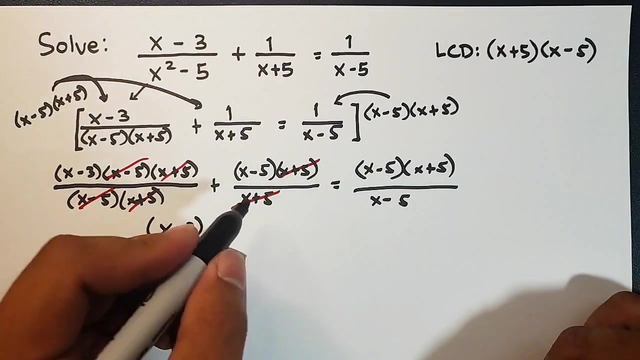 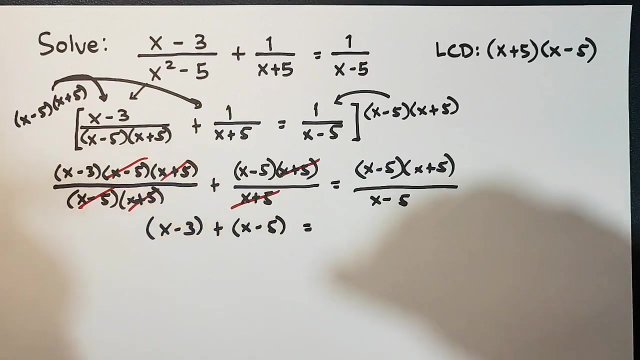 we can easily cancel out here: common common, common, common. so what we have now is simply x minus 3. plus this, you can eliminate x plus 5 and x plus 5. so what we have here is simply x minus 5. on the other side, we can cancel out: 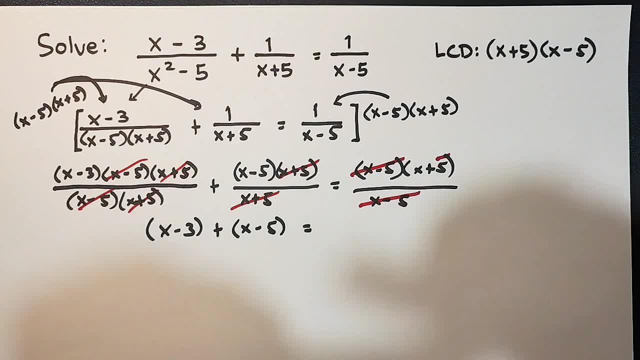 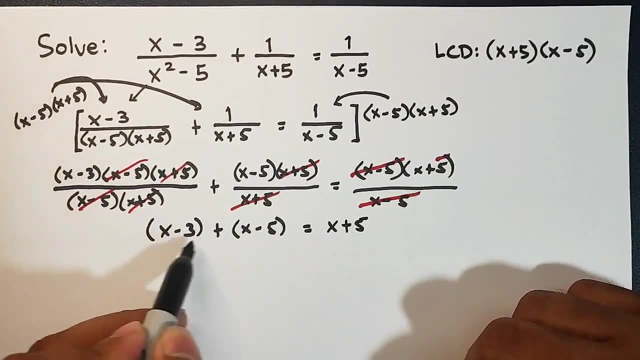 x minus 5 and x minus 5. so what will remain is x plus 5. so, as you can see, this will not multiply because it has an addition. let's just combine: x plus x is 2x negative. 3 plus negative, 5 is negative 8. 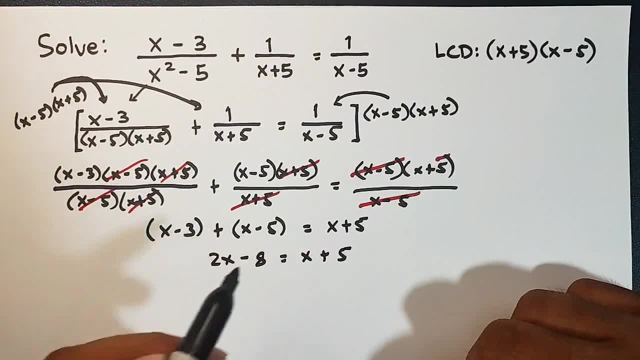 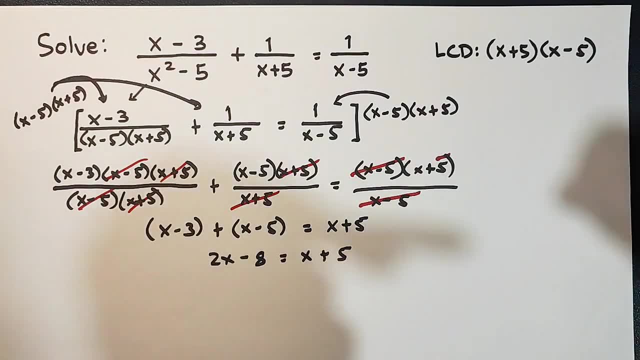 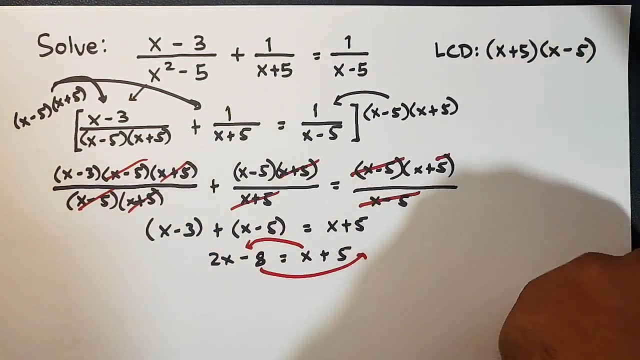 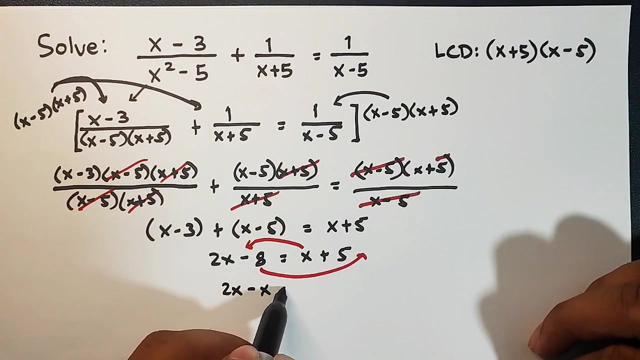 is equal to x plus 5. same scenario we will transpose again. we will transpose terms here our x will be transferred to the other side. this negative 8 will be transferred here. so we have 2x. transpose x to the other side. minus x is equal to 5.